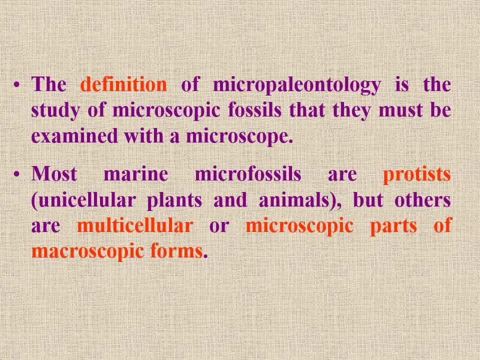 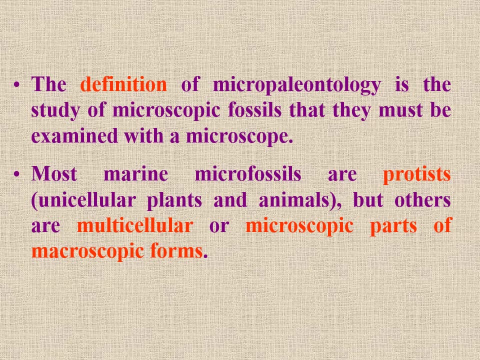 micro fossils which are examined under a microscope. most marine micro fossils are protist. that means they are unicellular plants or animals, but other multicellular organisms or macroscopic organisms that may be a part of the plant, that may be a part of the vertebrae. 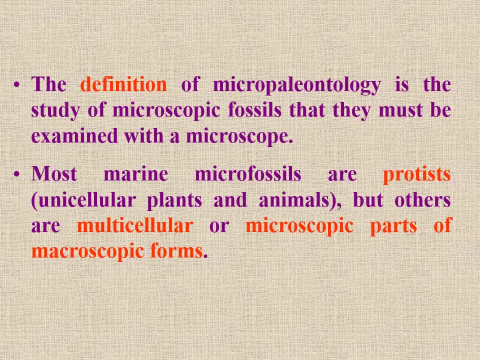 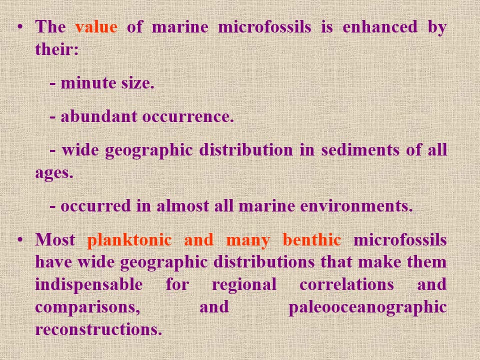 that may be a part of the invertebrates, but any macroscopic forms whose parts are studied under microscope, those are also deal in micro palaeontology. now, the value of microfossils, because we have learned the invertebrates, vertebrates, as well as the plants. so why the value of me microfossils? 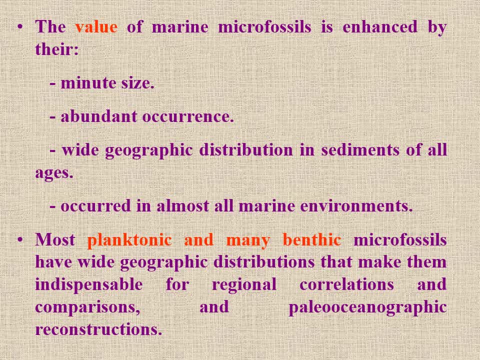 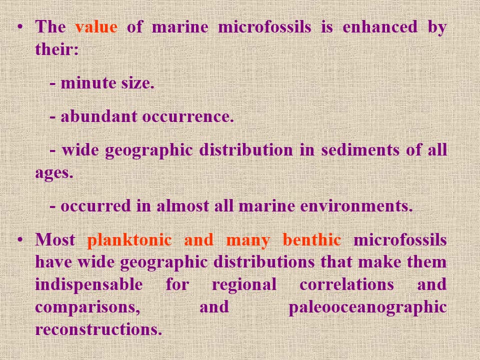 particularly the marine ones, how they help us to enhance our knowledge about the art, history and and same type organisms, now the micro organisms. they are minute or tiny in size, so they are very much not as big as the language to which we understand it, but they are Saxon. 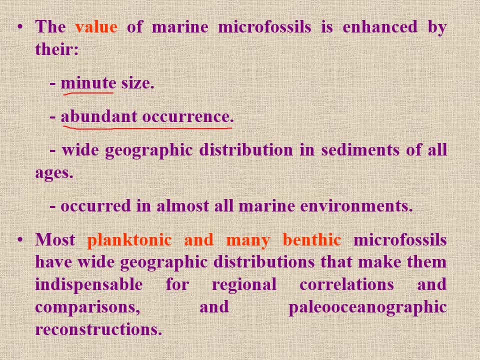 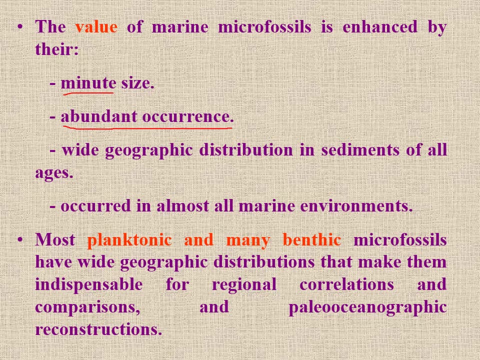 abundant in any kinds of sediments. suppose you go into the recent day beach area, in the recent day coastal areas and you take only a spoon of sediments, a spoon of sand. so within that one spoon of sand you may get hundreds or even sometimes thousands of microorganisms, the shells or dead shells of 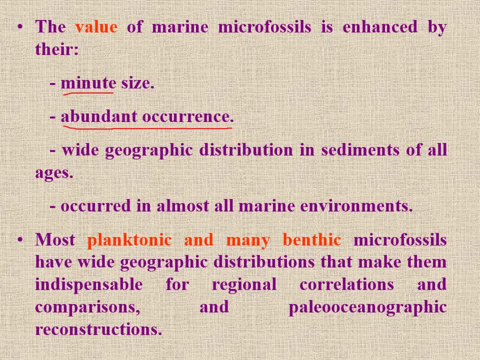 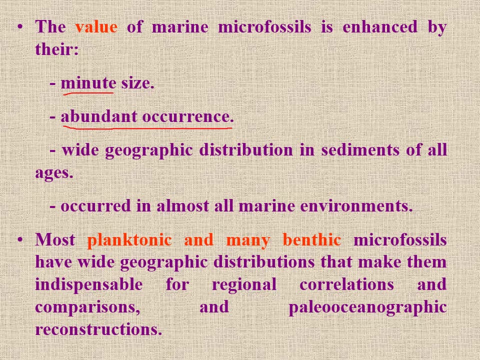 microorganisms, so you can have an idea that how much abundant are they just within a few amount or few volume of sediments. so because of their abundance we can easily get them in almost every kinds of sediments. now, the microorganisms they have, a wide range of. 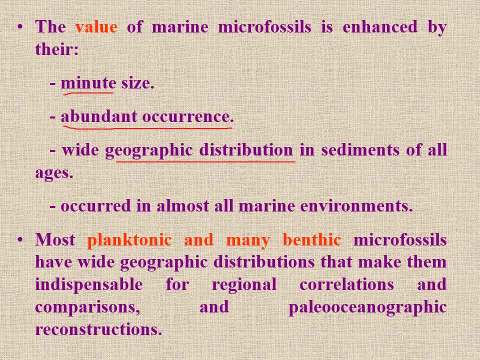 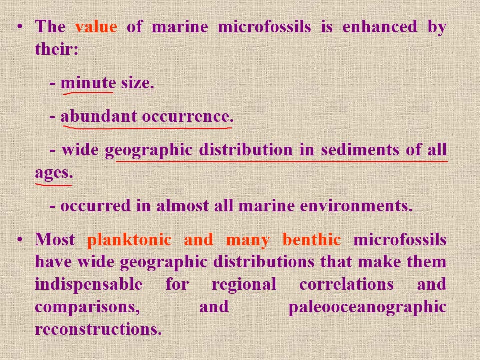 wide geographic distributions in sediments of all ages. so these microorganisms are found in the sedimentary rocks of all ages. so throughout the entire geological time we can study the changes or ups and downs, the morphological changes, the evolution changes of microorganism with time, with 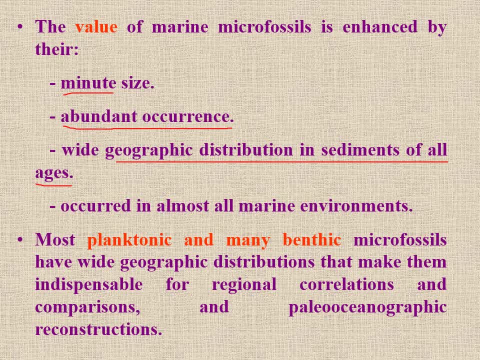 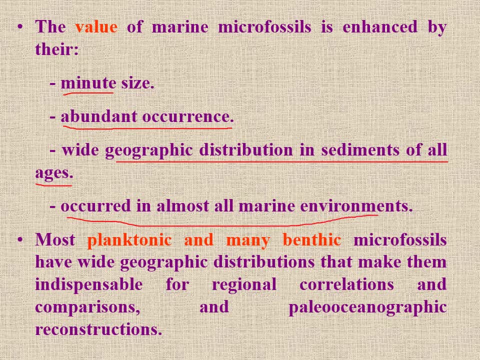 changing environments and they occurred in almost all marine environments. so any kinds of marine environments- it may be coastal, it may be shallow marine, it may be deep marine, even if they are also found in brackish water and sometimes they also found in freshwater environments. so any kinds of aquatic environments, these kinds of 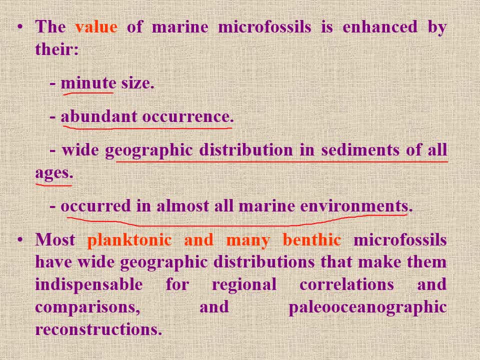 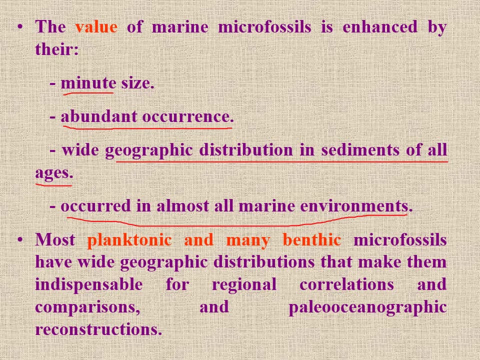 micro fossils and even in some terrestrial environments also specific kinds of micro fossils are founde, by which many kinds of geological work are easily done. and why we prefer- or why a paleontologist, ah, choose- the micro fossils because, as I told you, that they have very tiny or very min sven size. so the taphonomic, 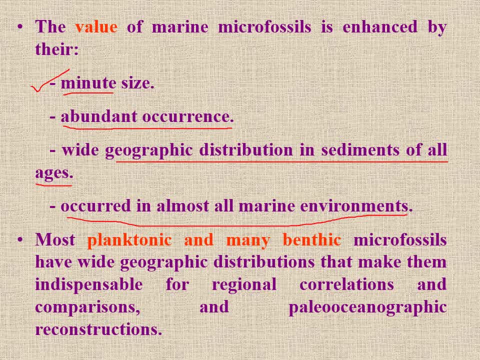 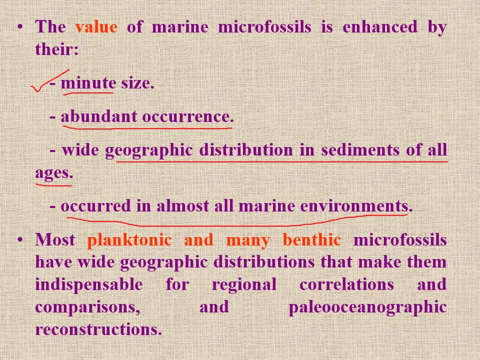 effect on these micro organisms compared to the macro organisms is very, very less, and that is why this will enhance their preservation. So we get ample amount of microfossils in almost all kinds of sedimentary rocks throughout the geological history. Now, most of the microfossils, they are either planktonic, 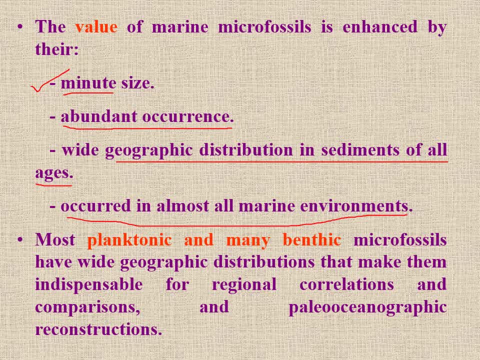 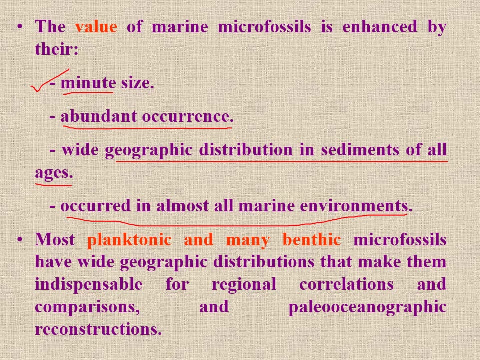 or benthic, So the micro organism above the water surface, above the aquatic body, and sometimes they are benthic. that means they are bottom dwellers and they are also vagile. that means they are moving, not fixed in a particular place, not sessile. 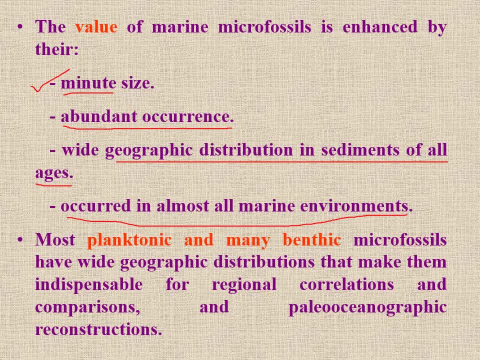 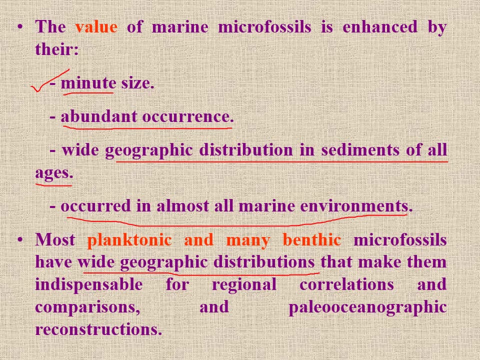 So being a planktonic or benthic microfossil, the microfossils groups. they have a wide geography, That means they are found in many parts of the world and this property helps a geologist or helps a paleontologist to go for global stratigraphic correlation on the basis of: 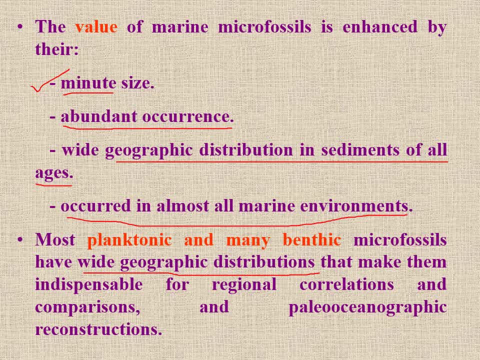 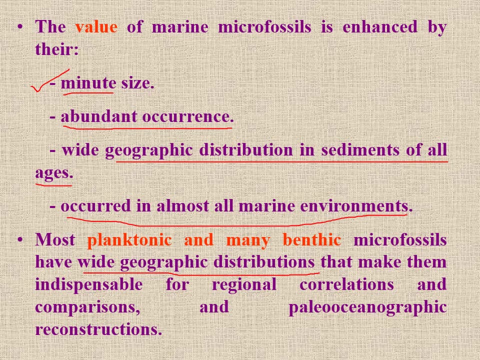 those microfossils, because we know from our previous biostatigraphic class that to do biostatigraphic correlation, the same kinds of fossil must have present in two different stratigraphic horizons which are separated vastly, So without the presence of same 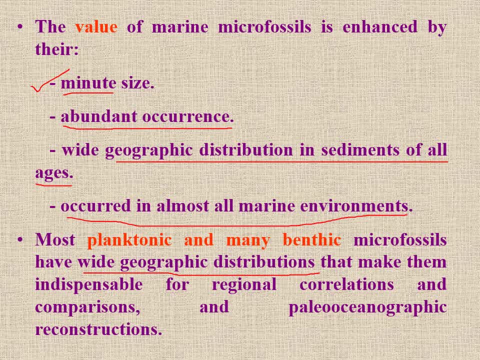 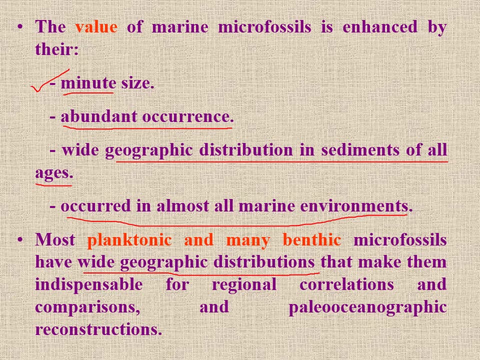 microfossils. we cannot correlate or you can say, without the presence of same kinds of fossils it may be micro or it may be macrofossil. also, And as microfossils have minute size, very abundant, they have wide geographic distribution. So these are the very good characters of an potential index. 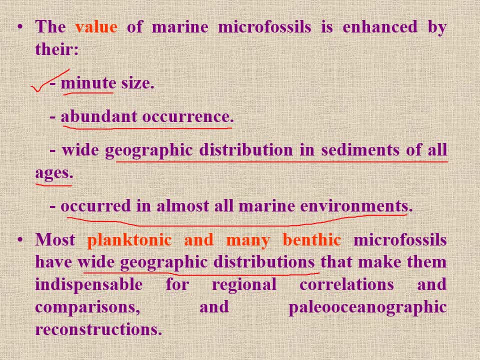 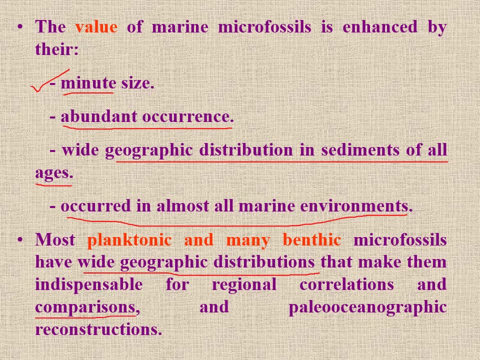 fossils. So with that we can easily go for stratigraphic correlations of different stratigraphic sections And on the basis of that we can also make some comparisons between different sections. that is, how sea level changes, how the environmental changes between two localities. 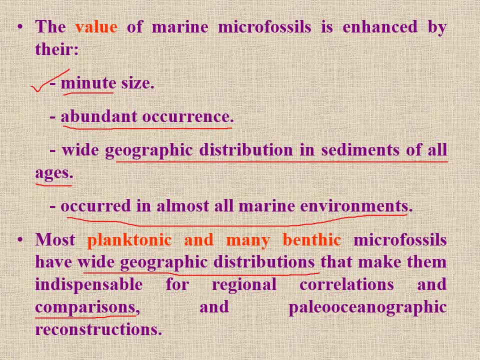 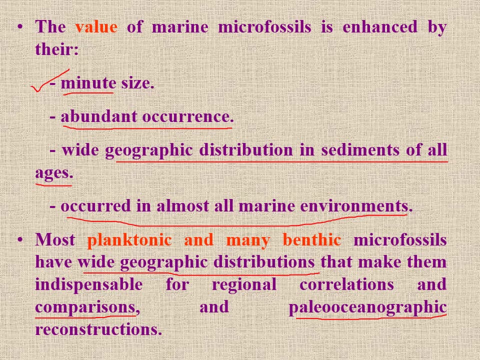 between two stratigraphic horizons and also paleo-oceanographic reconstruction, that is, the paleo-biogeographic reconstruction. So we can have an idea about the oceanic distributions. what are body of ocean surfaces, how they distributed in ancient time, based on the microfossils presence or absence. 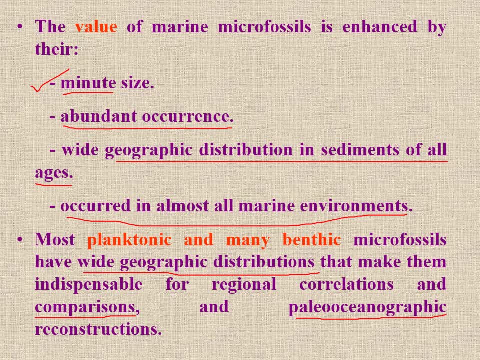 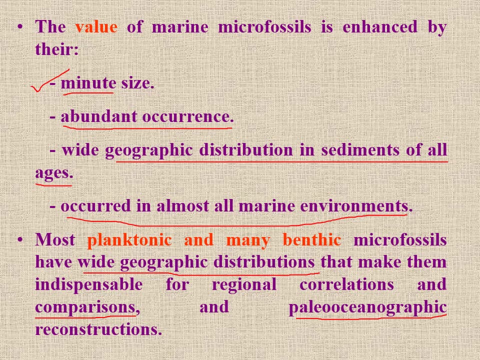 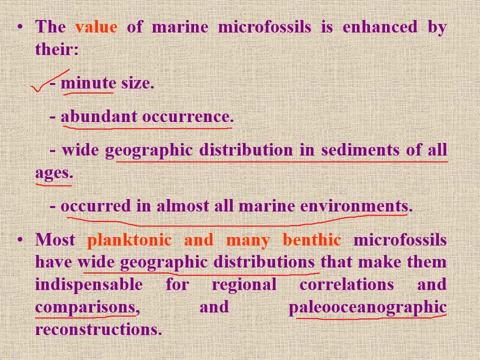 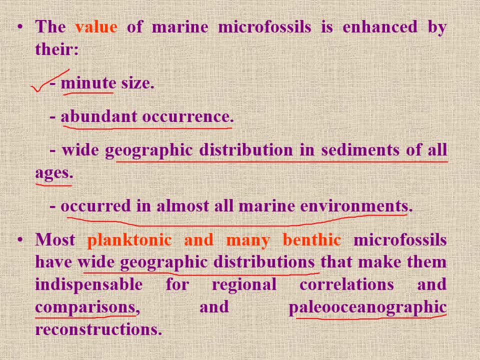 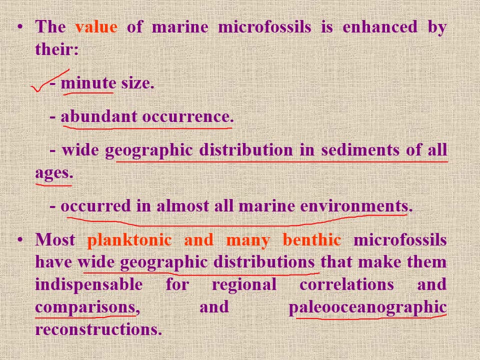 other important term is a Coronavi schedum, jedn, g, j n, c u s, or precisely about the aquatic bodies, about the oceanographic distributions in ancient time, So not only in correlation or in getting an idea about the ancient climate, but microfossils. 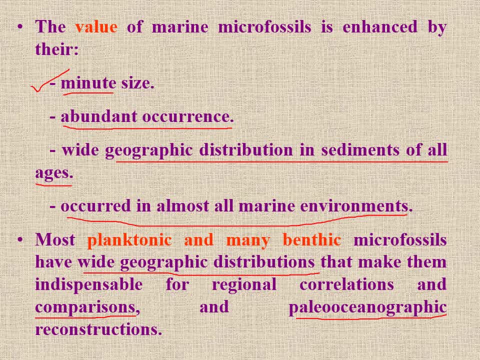 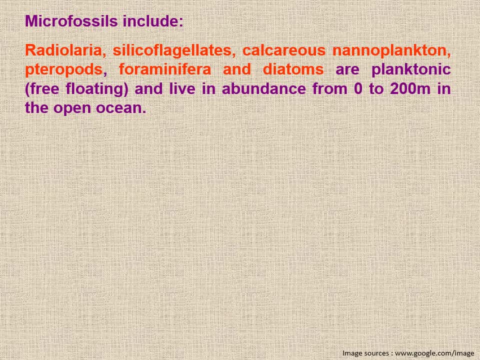 also helps us in paleo-biogeographic, particularly paleo-oceanographic, reconstruction. Now, microfossils include the radiolaria, silicoflagellates, calcareous nanoplanktons, pteropods, poraminifera. 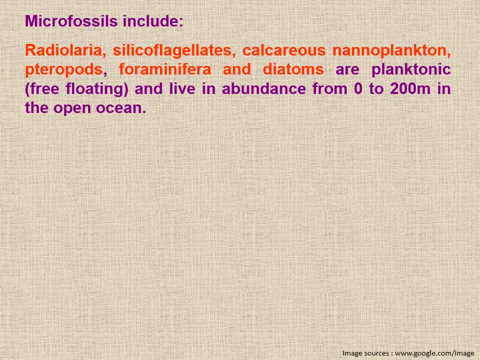 and diatoms And all these groups. they have planktonic life habit. That means they are floating within the water surface. They are highly abundant, From 0 to 200 meter, that is, within the photic zone up to which sunlight can penetrate within. 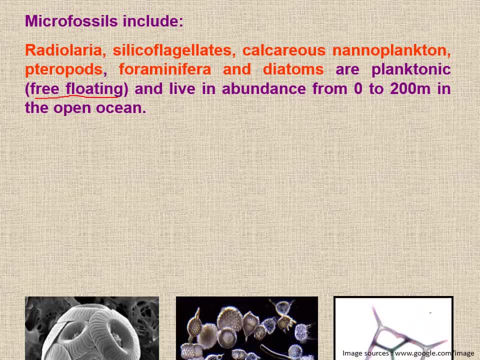 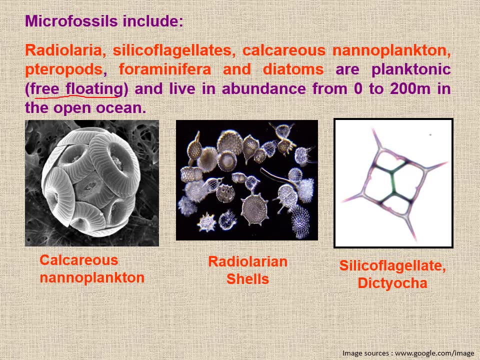 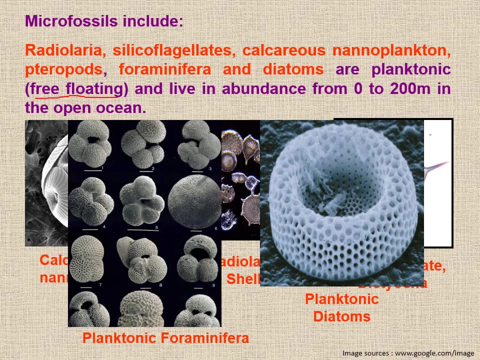 the ocean water surface. These are some pictures of the different planktonic microfossils, the calcareous nanoplanktons, radiolarian shells, silicoflagellates, Planktonic foraminifera, planktonic diatoms, and appreciate how much beautiful they are. 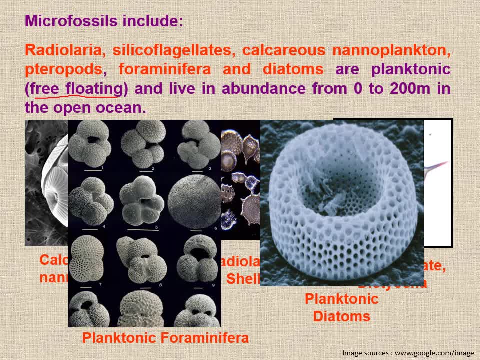 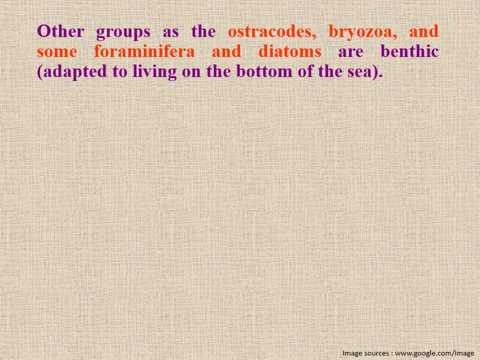 Although they are very, very tiny in size, but their shell structure, their hard part is looks amazing when we are going to observe them under microscopes. Other group of microfossils are also there. They include the ostracodes, the parts of briozoa. 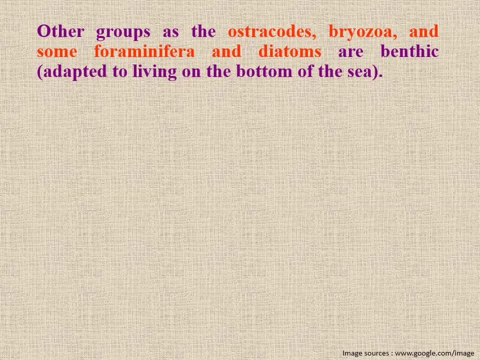 They are very, very tiny in size. They are very, very tiny in size. They are very, very tiny in size, But it is still very, very beautiful. But it is still very, very beautiful. And some foraminifera which lives in bottom surface. 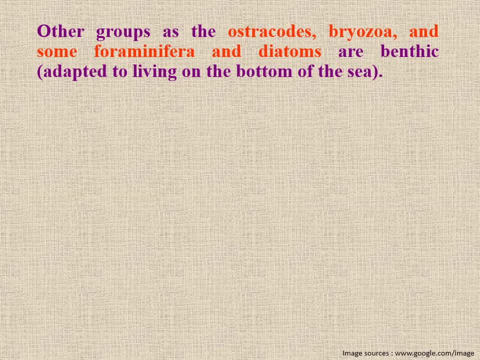 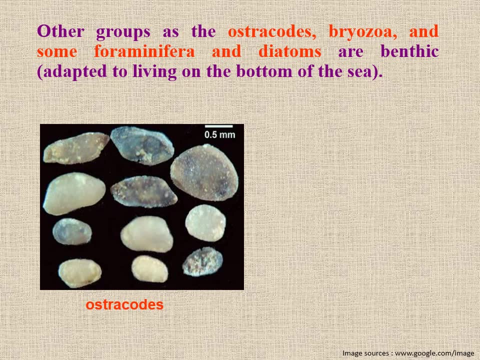 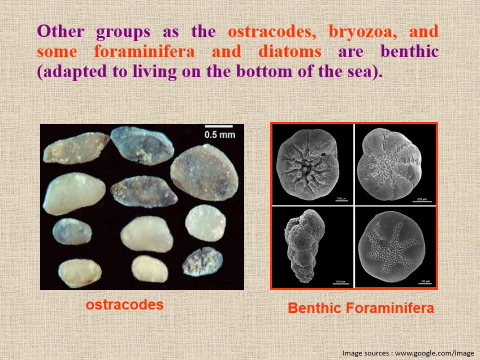 And some diatoms also, which have benthic life habit. That means they're living on the bottom of the sea. Here the ostracodes look like a tiny bivalve And these are the benthic foraminifera. 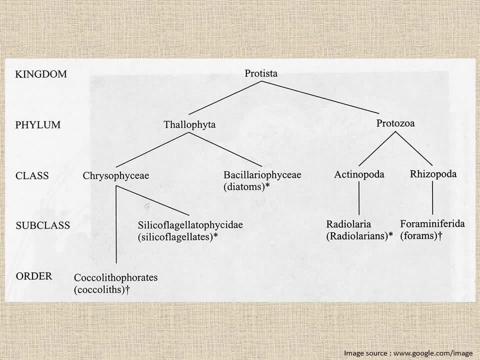 Now, If we look at the mixture phylogenetic classifications of microfossils or microorganisms groups, as i already told you that the microfossils belong to the means, all the microorganism belongs to the unicellular group and the protista kingdom is divided into two: phylum thalophyta and 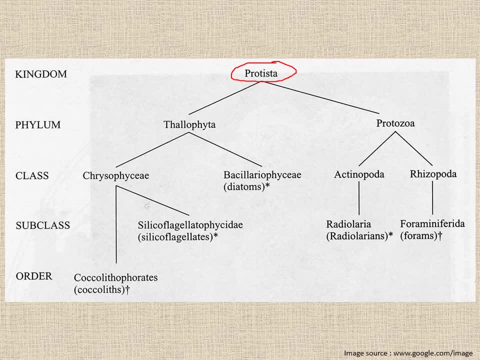 protozoa thalophyta phylum is divided into two class: cryophyche and bacillariophyche. these are the basically diatoms, and cryophyche again is divided into one subclass and one order. the order is coccolithophorates. subclass is silico flagell to phi, cd and the protozoa group. 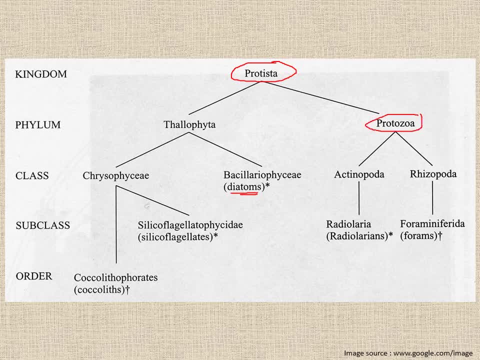 this group is divided, or this is divided into two class: actinopoda and rhizopoda. actinopodas are the radiolarians and rhizopoda are the foraminiferida. now, within our undergraduate syllabus, we have to only study about the detailed morphology, cell morphology and characteristics of 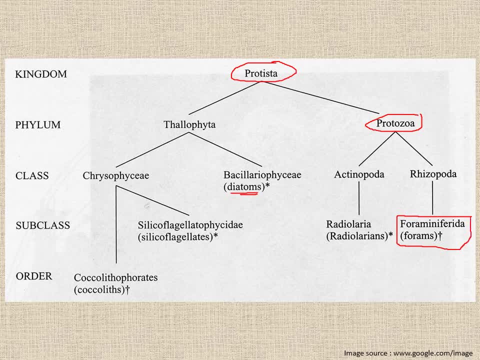 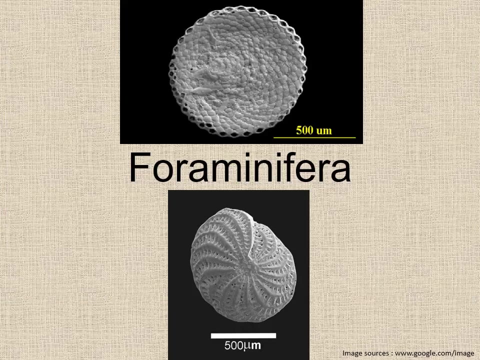 the group foraminiferida, that means the forums. this forum names is a nickname, so it is known as the subclass foraminifarida, or even we know them as foraminifera, and it is nicknamed as forums. now here are the two beautiful pictures of foraminifera, how they 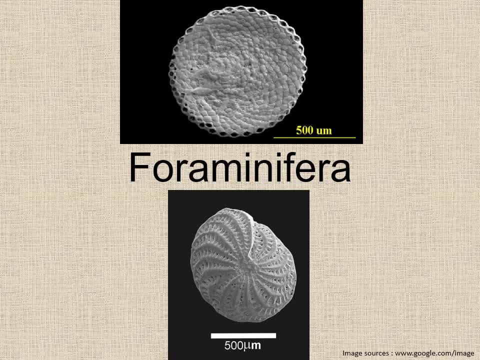 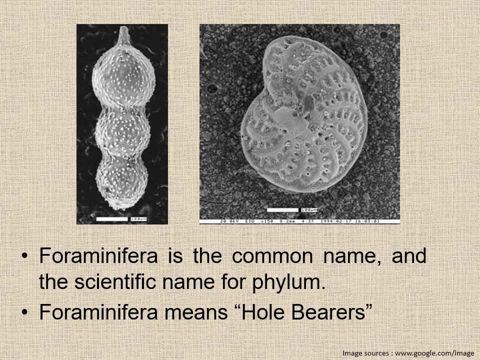 looks. so here you can see a flat dis zeped foramini ferry and in this picture you can see a coiled foraminifera. now if we look at the nomenclature of the group, so it is the foraminifera. it is also used as the common name from the group, or it is also: 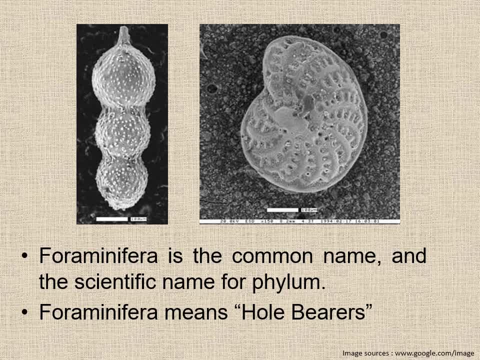 the scientific name of foreign taxonomic group, that is, the phylum. so both scientific name of the group and the common name of the group are same, and that is foraminifera. now the meaning of foraminifera term is hole bearers, as the 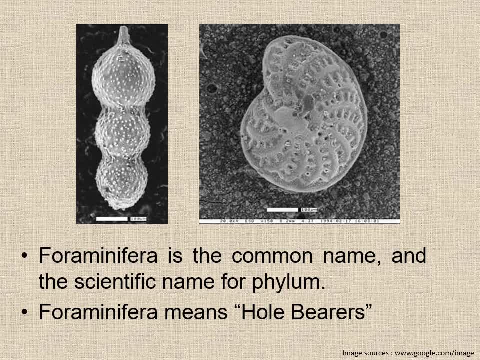 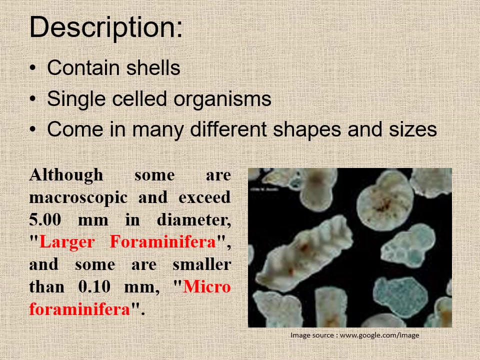 foraminifera consists of numerous numbers of holes, so that is why these group of organisms are known as foraminifera. that means hole bearers. now, whom we called foraminifera? or what are the characteristics of foraminifera? as I already told you, these are protists. that means they are single-celled. 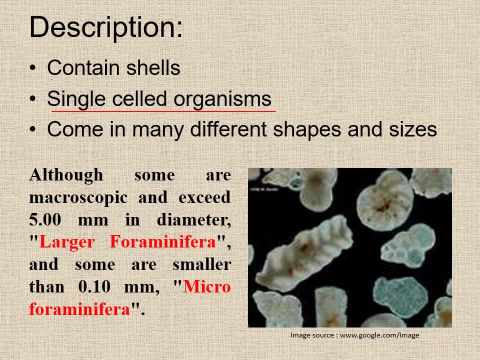 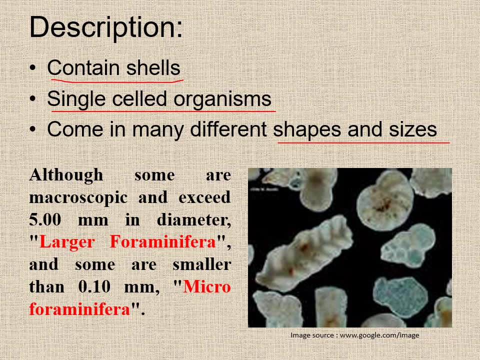 organisms. they have hard parts, that means they have the skeletal part, contain cells and they may come in different shape and sizes. so, although some of the foraminifera- or, as I, as we learn from the previous slides, that foraminifera is a group under microorganisms and all microorganism, 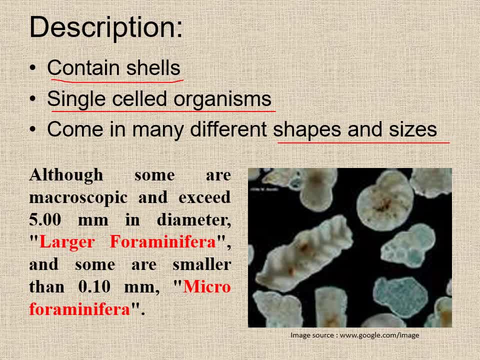 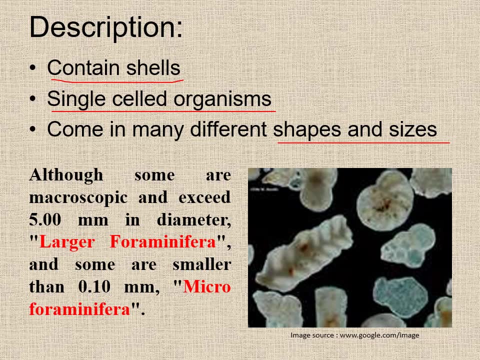 means that means they are studied under microscope. so foraminifera are also smaller organisms which are observed, which are studied under microscope, and most of the foraminifera they are very tiny in size, often less than 0.10 millimeter. we call them as micro foraminifera, but 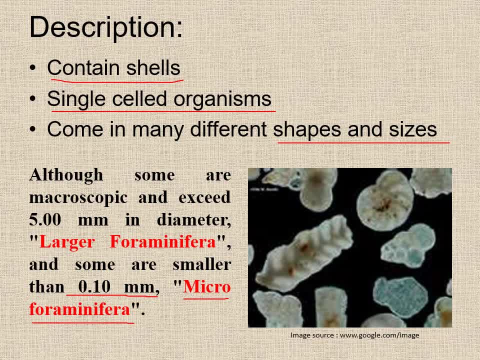 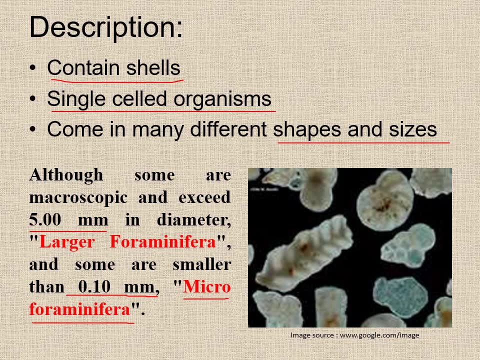 there are some foraminifera cells or some foraminifera hard parts found in nature which have the diameter exceeding 5 millimeter, almost a 50 paisa or 1 rupee coin. so those larger sized foraminifera which are macroscopic, that 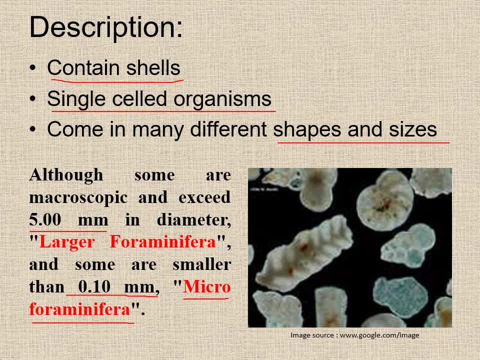 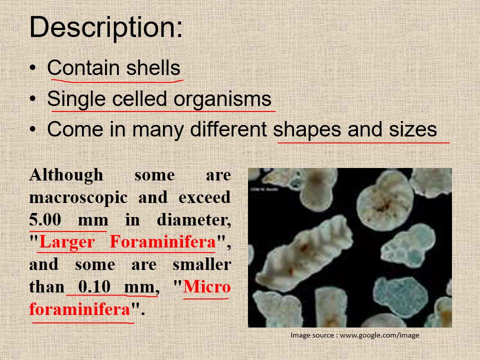 means they can be identified or they are very much visible to naked eye. those are known as large sized foraminifera- larger foraminifera, so it's simply based on size. those having diameter 5 millimeter and above those are larger foraminifera and those are observed. 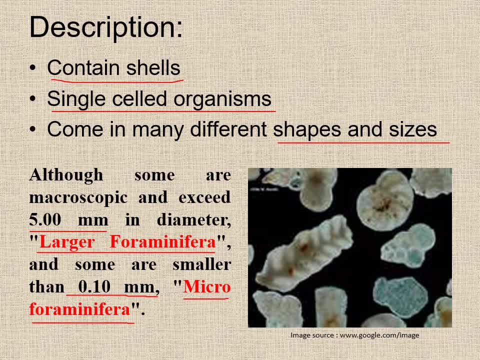 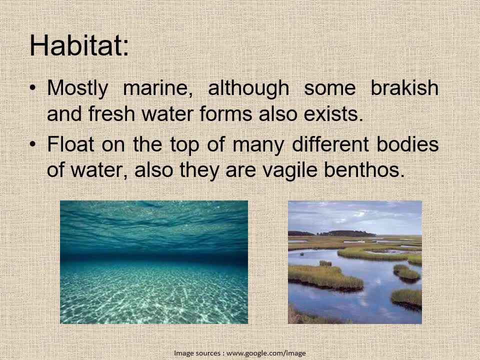 under microscope, mostly less than 0.1 millimeter. those are known as micro foraminifera. now come to the habitat of foraminifera. they are mostly marine, living in almost all kinds of marine environments, like the shallow water, deep water and deep water. 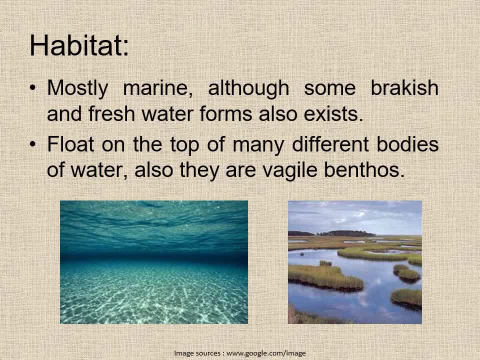 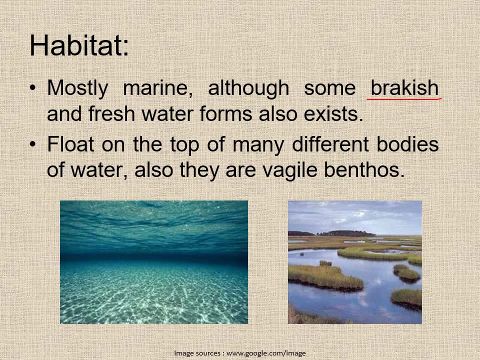 deep water, coastal area, deep sea, any kinds of marine environments- foraminiferas are found. not only that, they are also found in brackish water. that means it is a place where the marine water meets with the fresh water, and even they are found in some freshwater conditions also. so you can see that foraminiferas are. 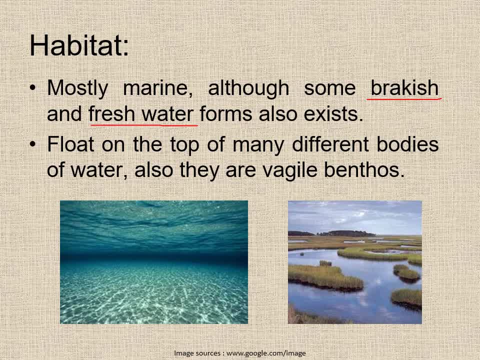 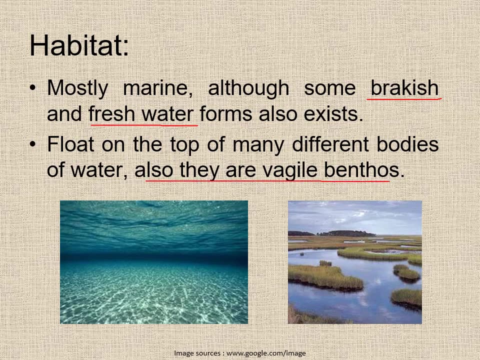 almost found in every aquatic conditions. foraminifera float on the top of many different bodies of water, that is, they are planktonic and sometimes some foraminifera. they are also agile benthos. that means they live in the bottom substrate, in the bottom surface. 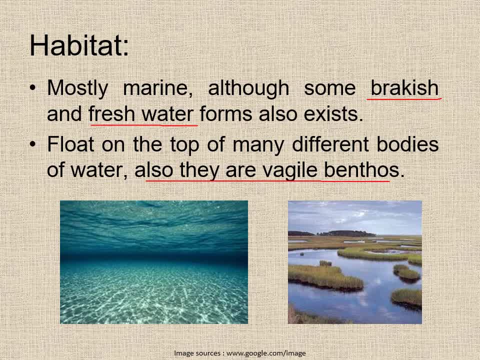 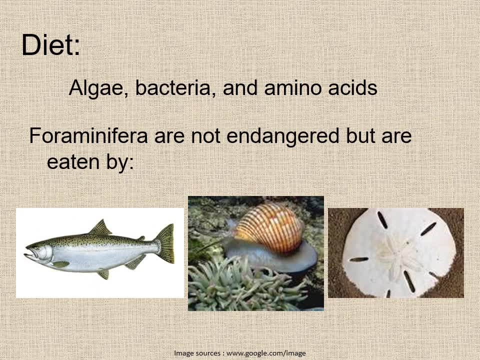 of water and they can move also. now what foraminifera eat? mostly, foraminifera eat the decomposed algae. foraminifera eat the decomposed algae bodies, bacteria and the amino acids parched in the sea floor or within the water surface, and foraminifera are eaten. 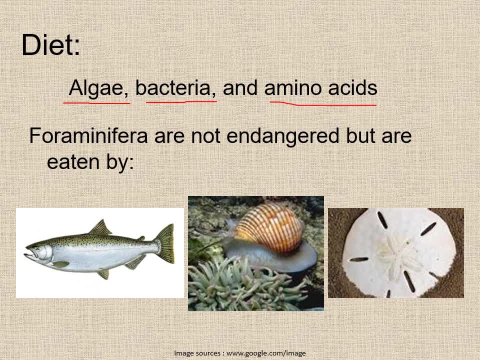 Algae bodies, bacteria and the amino act. seeds dispersed in the seafloor or within the water surface and foraminifera are eaten by the fishes, gastropodes and Gastropods and a kenoids, so these organisms take foraminifera as their food. 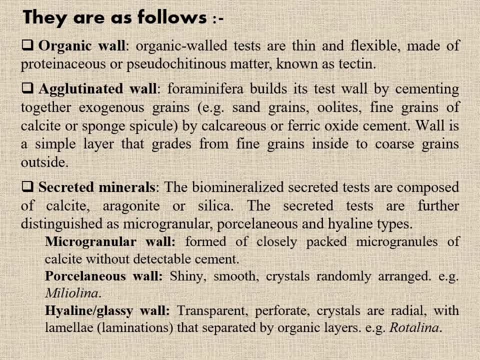 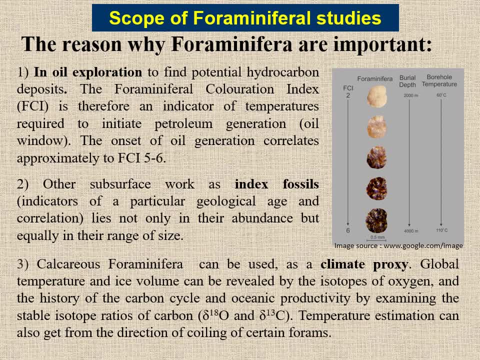 material which are found in nature. now why we study the foraminiferous. that is the scope of the foraminiferous studies. the reason of foraminiferous study are many in numbers they have a lot of importance, particularly in the study of the hydrocarbon, that is, for the oil sector study, that is, those people's which 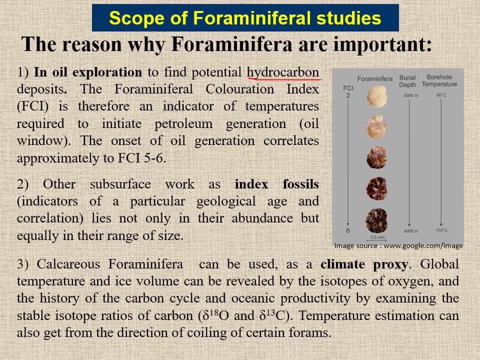 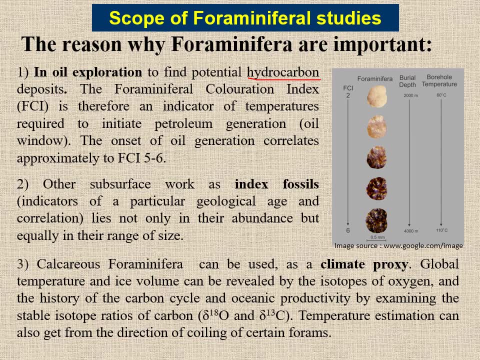 who try to find the subsurface occurrence of any hydrocarbon, the subsurface occurrence of any natural oil, how they will identify that any place is a potential place for oil generation, because they depend on the foraminiferous color index, which is abbreviated as fci, now as foraminiferous deposited within the aquatic. 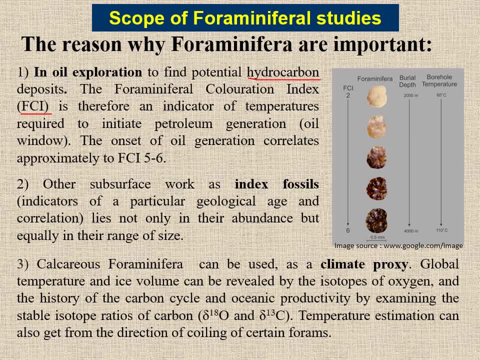 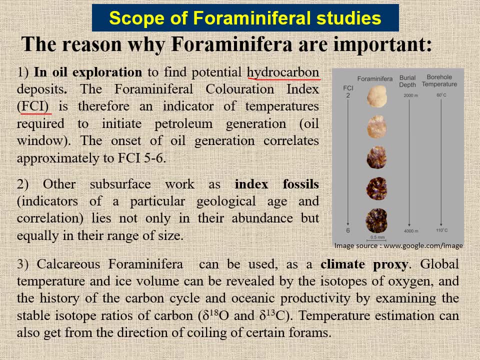 bottom, that is, within the substrate, and time after time they are covered with another time sediments. so gradually, those foraminiferous cells, those foraminiferous taste will go deeper and deeper and, as we know, with depth the geothermal gradient is also increasing. that means the temperature pressure condition is increasing with. 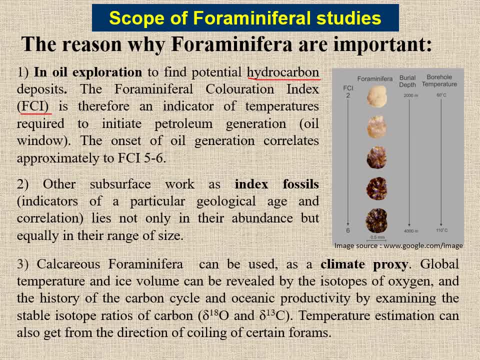 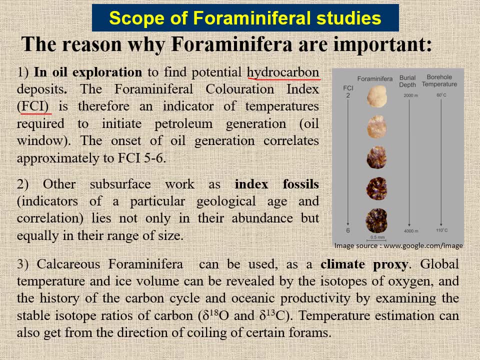 depth. so as the sedimentary deposition goes below and below, that means they are covered with more and more sediments. they will feel more pressure and more temperature. now, with increasing pressure and temperature, the forum peripheral taste will also changed. with this increasing pressure, temperature condition, particularly the color of the foramini feral test is changed. you can see here is a. 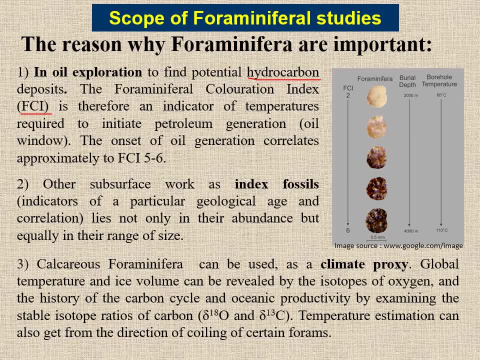 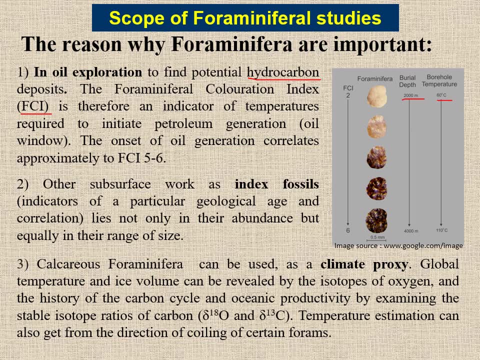 broad graph showing the different color change pattern with depth and with increasing temperature. so you can see a photominiferal test at about 2000 meter depth and about 60 degree centigrade temperature it looks like white, whereas with increasing depth the photominiferal depth becomes more darker and darker. so at 4000 meter depth, 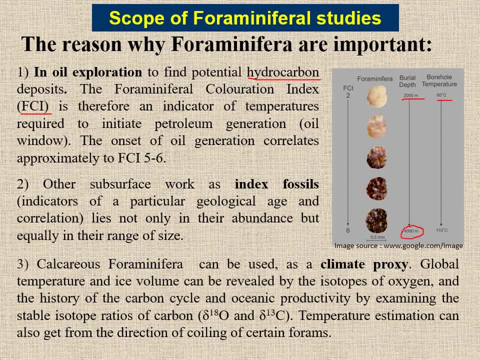 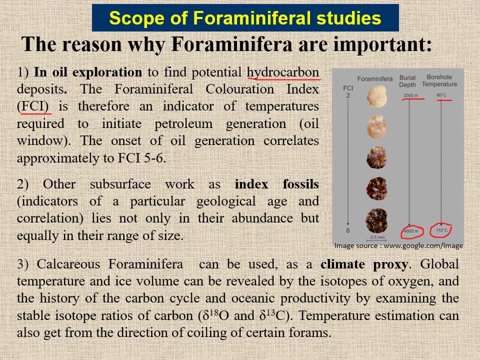 just doubling the depth, where temperature is about 110 degree centigrade, the photominiferal test become extremely dark. so accordingly micropaleontologist or oil sector geologists, they divide this color skin or different colors of photominiferal test into a photominiferal coloration index. so here it is for fci two. fci three: 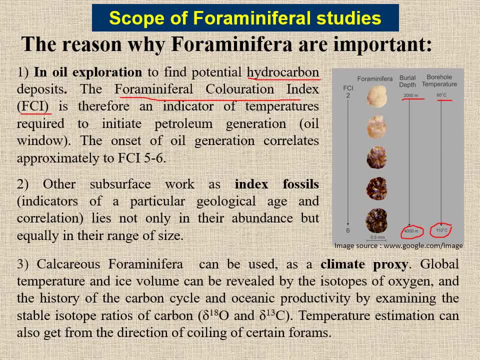 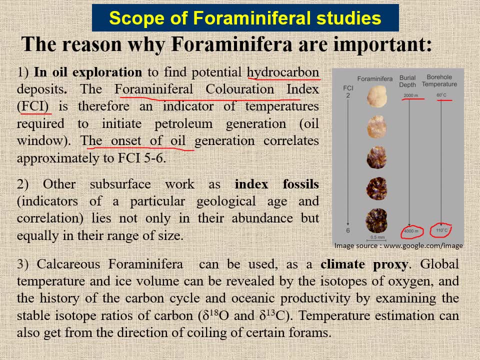 four, five and six, so more and more dark color of photominiferal test we get in the sedimentary rock record. that means they have suffered more and more pressure and temperature and the onset of oil generation is correlatable with the photominiferal color index of five. 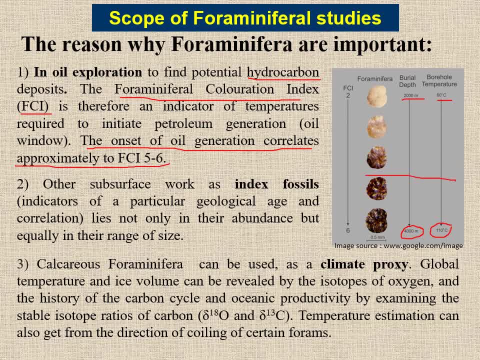 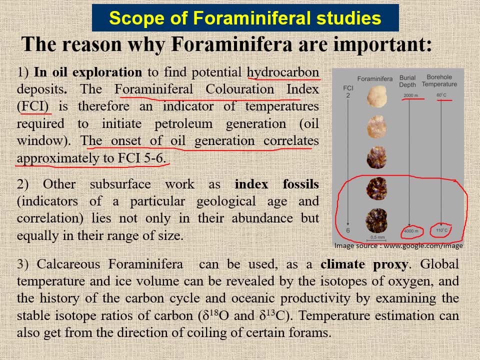 and six. so in this pressure, temperature depth, that is the suitable condition in which we can expect that that area or that sedimentary deposition is going through the generation condition of natural oil or hydrocarbon. so whenever from the surface rocks, palen-, micro-paleontologists or 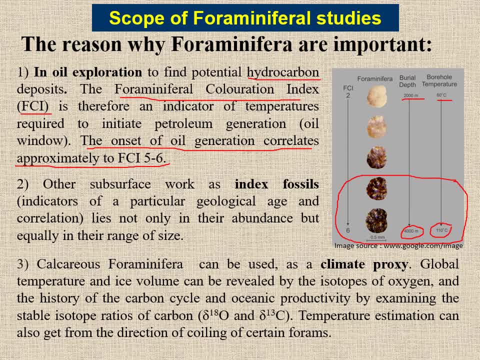 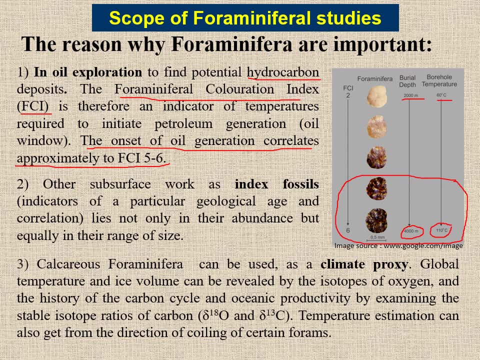 paleontologists get these photominiferal tests having the FCI five or 6 eta abraha, They will go to study those rocks further because these are the potential deposits which have ample chance that there we get natural hydrocarbon deposits or they are the place. 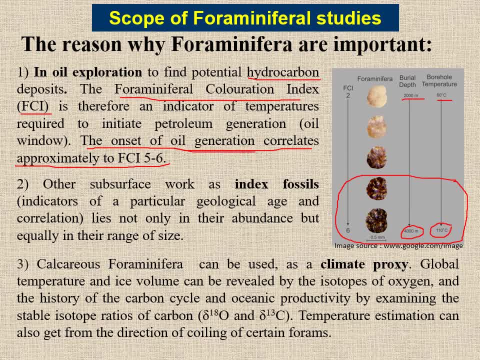 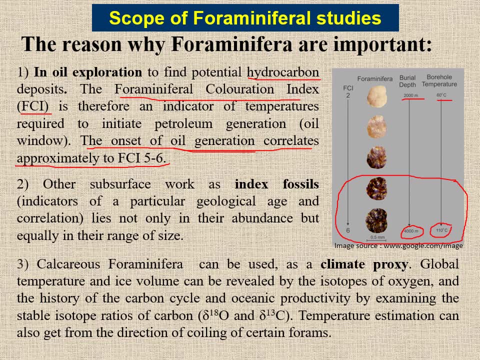 which will give you the natural oil in the subsurface rocks. Apart from the indication for oil exploration by the foraminiferous shell colours, foraminiferous shells are also used for any kind of subatomic graphic correlation in a global base because, as I already told you that foraminiferous shells are highly abundant, they are tiny. 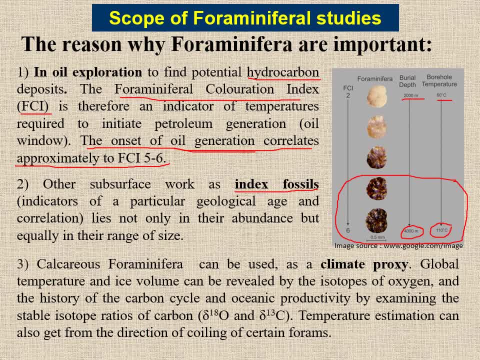 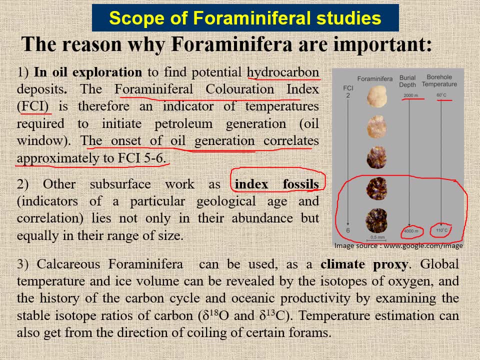 in size. they have a wide geographic distribution. So all these properties are satisfying that they have the characters for a good index fossil. So they are highly used for any kind of static graphic correlation studies throughout the global sections, Some calcareous, foraminiferous. they are also used for climate indication. 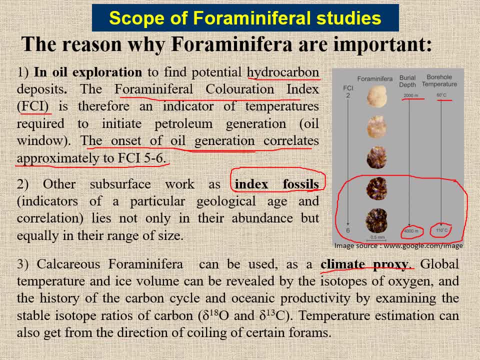 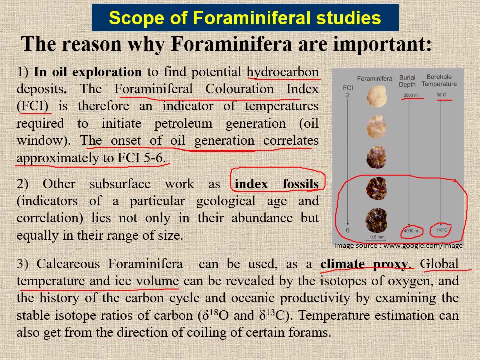 That means foraminiferous shells. they are very good tools for climate proxy. That means they are giving some climatic data of ancient time. Global temperature and ice volume can be revealed by the isotropic study If a foraminiferous shell is composed of calcareous material. 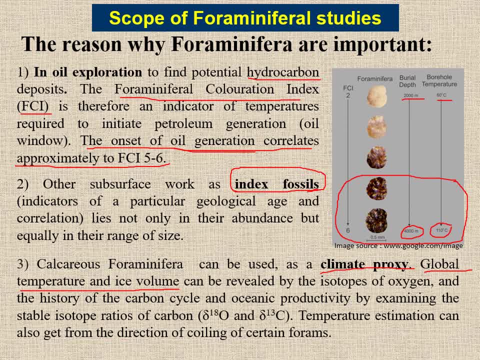 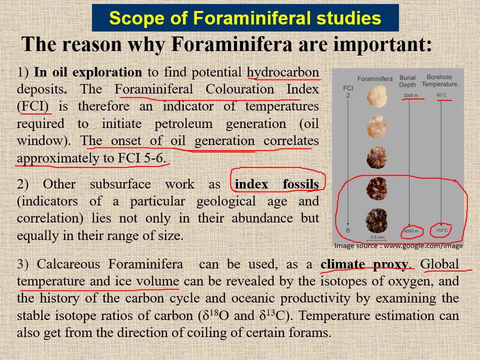 That is simply calcium carbonate. You can get the oxygen isotope, You can get the carbon isotope within those foraminiferous shells And, on the basis of the ratio between the heavier isotopes and the lighter isotopes of oxygen or carbon, we can get an idea about the temperature, about the oceanic productivity. 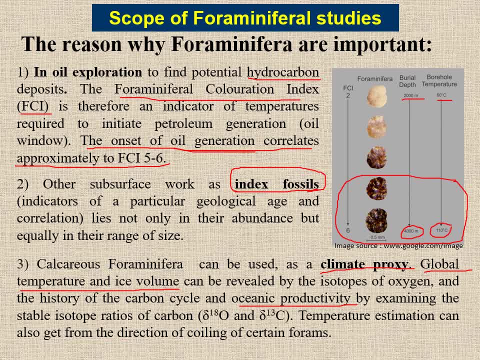 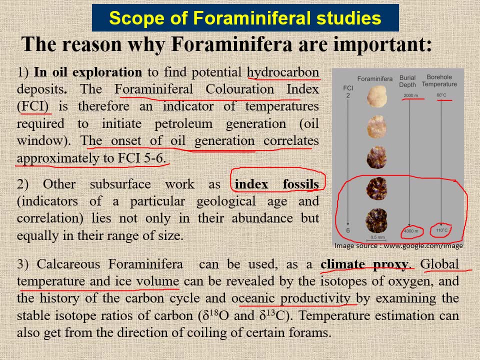 or about the sometimes the global circulation of that Of the oceanic water. So by isotopic study of foraminiferous taste we can get an idea about the global temperature or global precipitation condition of ancient times. Another very interesting thing by which we can get an idea about the ancient paleoclimate: 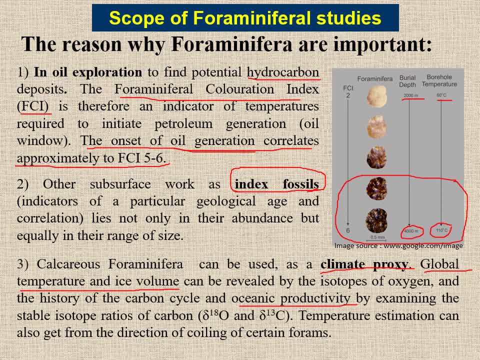 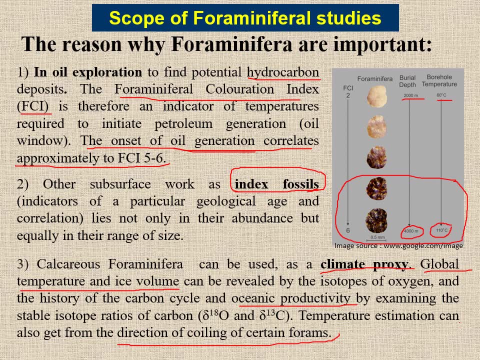 condition, That is, the direction of coiling of the foraminiferous shells. There are some foraminiferous which are very much sensitive to temperature And depending on that, they have changed their direction of coiling. So say, for example, in hotter condition, in high temperature condition, the foraminiferous 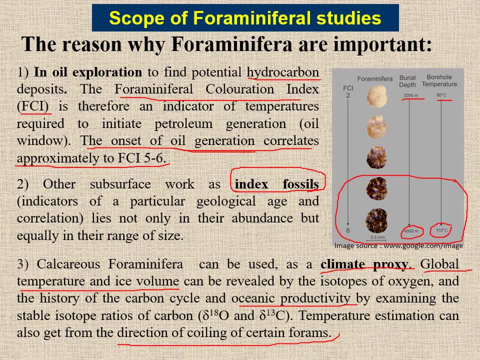 shell, Most of the foraminiferous individual of that particular species. They have changed their direction of coiling, So in the right hand coiling the foraminiferous shell of that particular species will go for sinistral coiling. 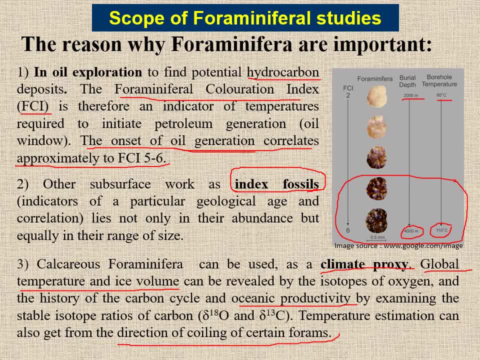 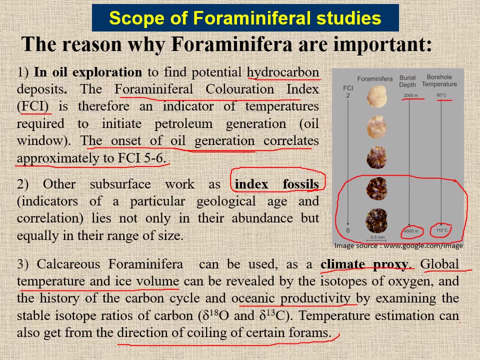 So, oppositely, for colder condition in cooler condition, the most of the foraminiferous shells of the same species will go for dextral coiling, That is right hand coiling. So with counting the relative abundance of dextral and sinistral coiling of that particular, 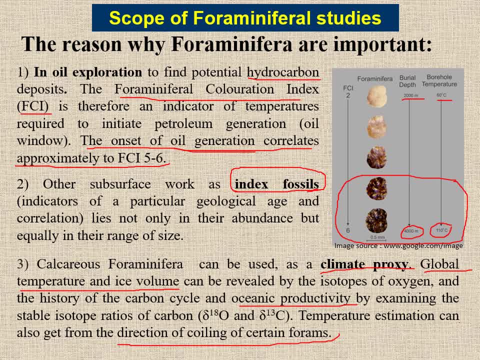 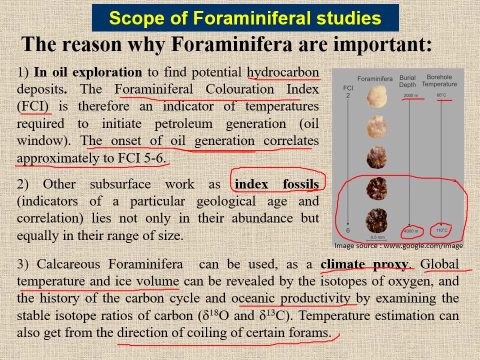 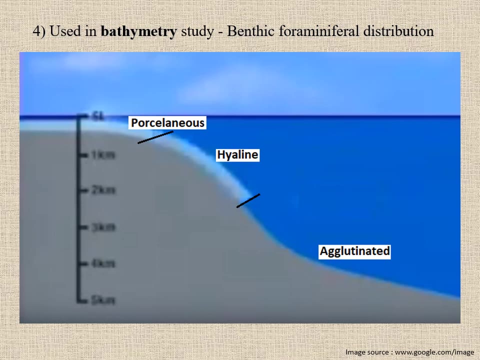 foraminiferous species. We can get an idea about the temperature species. we can get an idea about the broad temperature variation of any region, or even it can done globally also. next, foraminifera are also used. learn that the foraminiferal cells. 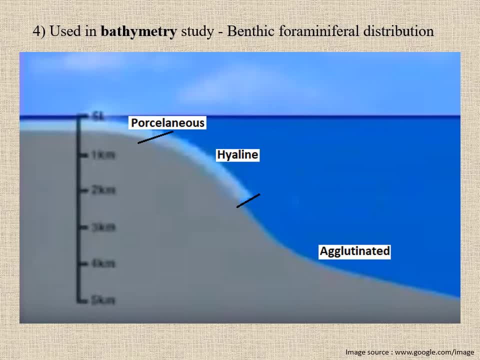 are made up of different material. some are made up of organic material, some are agglutinated, some are secreted material. so you can see that in a standard bathymetric profile, in a standard oceanic profile where you can get an idea about the change in depth of the ocean surface, of the 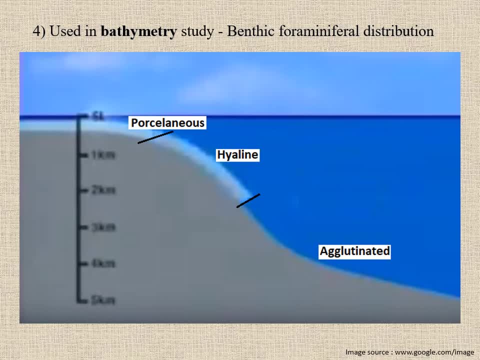 oceanic aquatic body, the how the benthic foraminiferal shell distribution or how the benthic foraminiferal distributions varies with depth, with bathymetric dan them. so in the salwar conditions, that means mostly in the selfal area, mostly near the coastal areas. 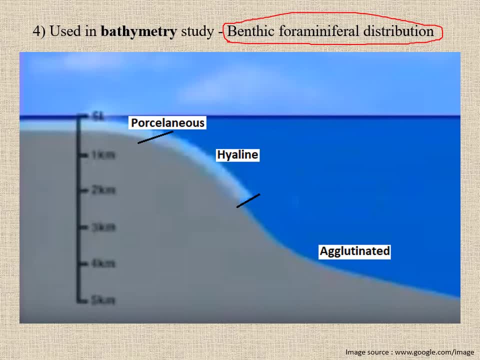 most of the Benthic Foraminiferal tests are porcelain as in composition, whereas in relatively deeper depth, that is, in moderate depth, the banka foraminiferal cells are of hyaline type and, in further deeper condition, in depth of oceanic body, at about three kilometer to five kilometer, most of the benthic foraminifera 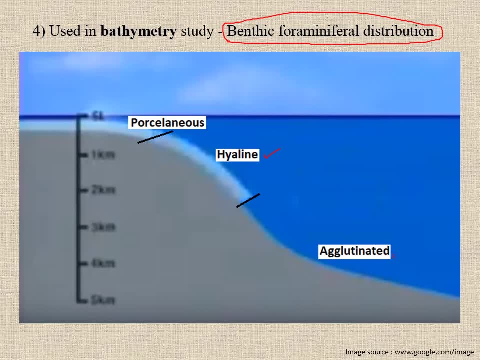 cells are of agglutinated type. so just by observing the relative abundance of different test material, of foraminifera, we can get an idea about the relative bathymetry, that is, the relative depth of ocean columns where we get those foraminifera test. another study by which we 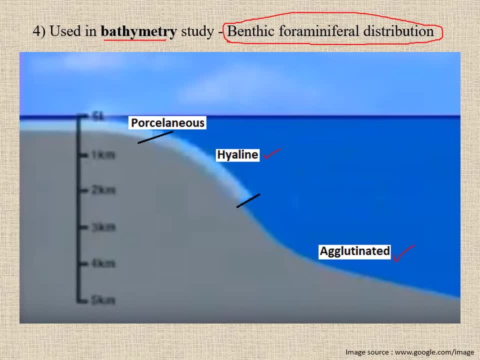 can get an idea about the planktonic is to benthic ratio. that means if we count the any deposition, because the planktonic forms are floating on the water surface whereas the benthic benthic forms lives above the substrate. so after the death of the organism, the benthic, 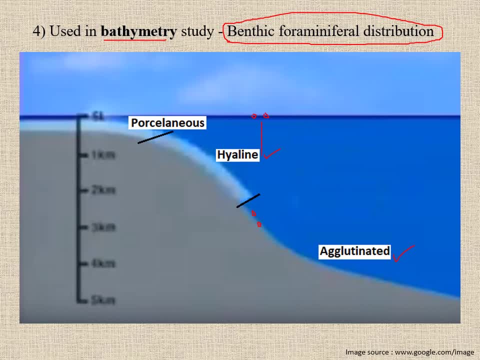 form remains here and the planktonic forms settle on the oceanic surface. so after the death of any individual, we get both the planktonic forms and the benthic forms together on this bottom substrate. now, if we collect all the planktonic and benthic forms with depth of 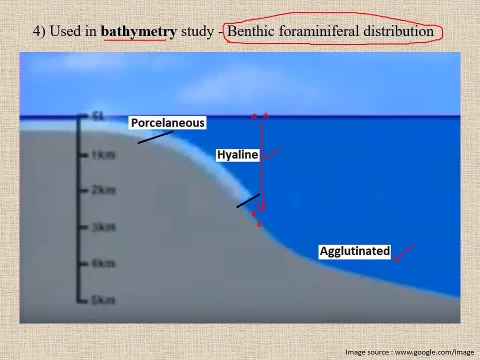 the ocean columns and we get a ratio of planktonic forms. planktonic foraminiferas is to bendic foraminifera. we can see that the ratio will be higher as we move from coaster to deep sea. so planktonic x benthic, this ratio will be higher than the dip crecigial好好. 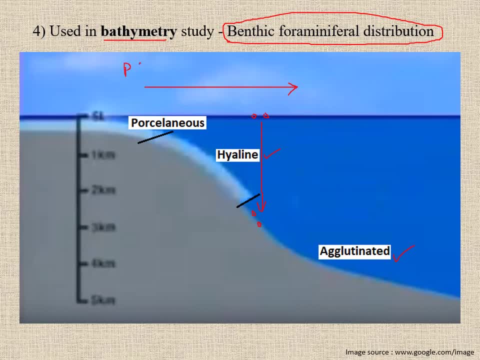 so this is the ratio we can get. this ratio will increase from coast to deep sea. Now the question comes why it occurs. The reason behind is that the planktonic foraminiferal distribution is largely controlled by the temperature, pressure, density of the water, salinity, oxygen condition and other chemical. 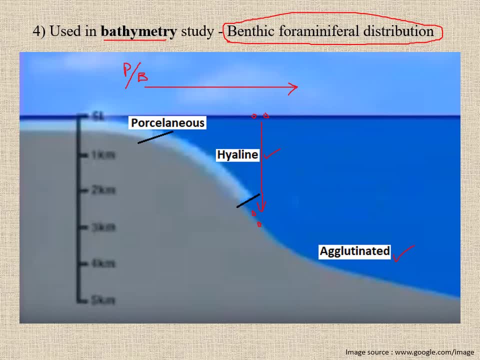 or biological factors. So, among these, the salinity and turbidity of the water, of this marine water, that will restrict Or that will decrease the salinity of the water. So, among these, the salinity and turbidity of the water, of this marine water that will. 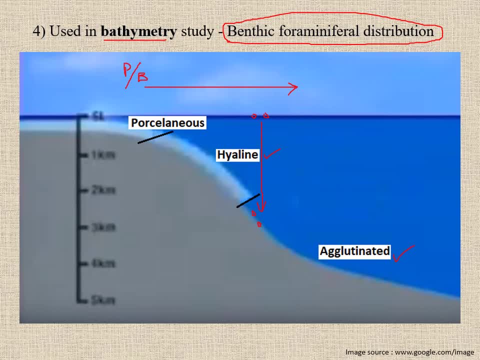 restrict Because of the redundancy of water throughout the presentation. So along with the salinity we have another part of the sheet in the encontrar distribution areas where wave activity, particularly the breaking of wave, is mostly found. So there is a regular churning of the entire water column and marine sediments. 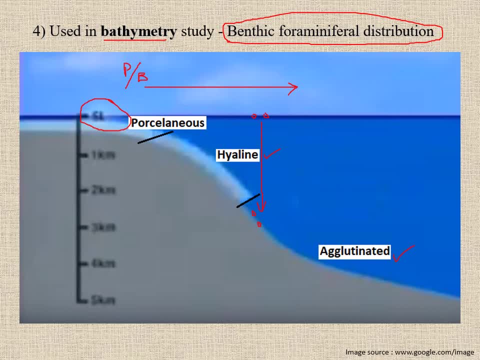 So this water becomes highly turbid. So because of these two reasons- the low salinity and highly turbid condition in the coastal areas or near coastal areas- that will restrict the abundance of planktonic foraminifera, Whereas as we move from coastal areas to the deeper part or to the open ocean, there the 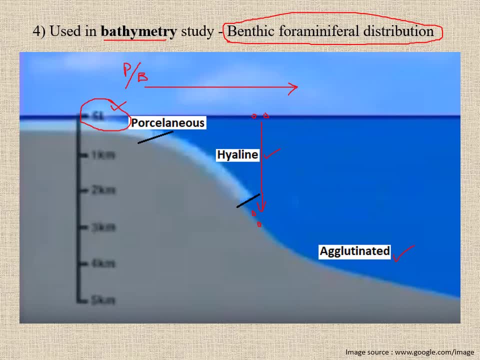 ocean water is calm, salinity condition is high compared to these coastal areas. So in these areas we will get higher numbers of planktonic foraminifera. Now, if we consider that the number of babies In thick polyph потому say, for example, the number of benthic foraminifera is constant, 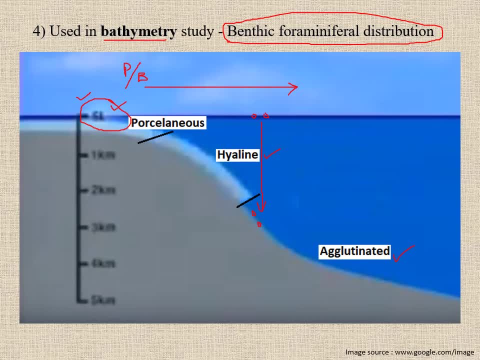 throughout the different date. Say, for example, number of benthic foraminifera in this area is about X. Here also, the number of benthic foraminifera is X. the number of benthic foraminifera And here also the number of benthic foraminifera is X. 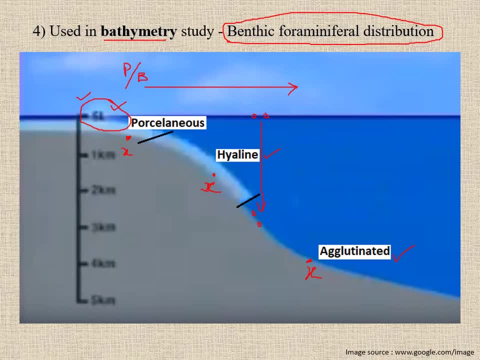 Now, in coastal areas, say, for example, the number of planktonic foraminifera we get is y1, here, in this condition, the number of planktonic foraminifera is y2 and in this condition in the water surface above the water surface, 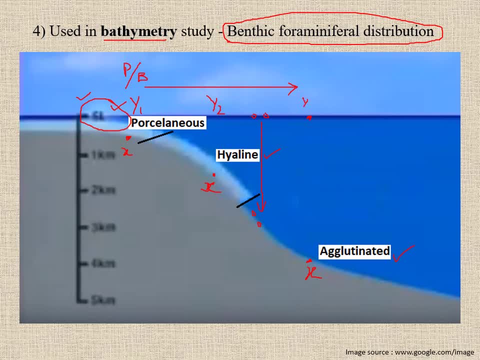 the number of planktonic foraminifera is y3.. So if we go for the ratio of planktonic and benthic foraminifera in these three depositional condition after the death of the foraminifera, we get a ratio here at this point. that means 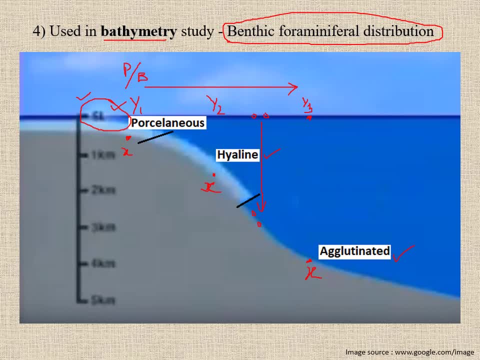 near the coastal area as y1 by x. In this condition the planktonic is to benthic foraminifera ratio is y2 by x, and here the planktonic by benthic foraminifera ratio is y3 by x. 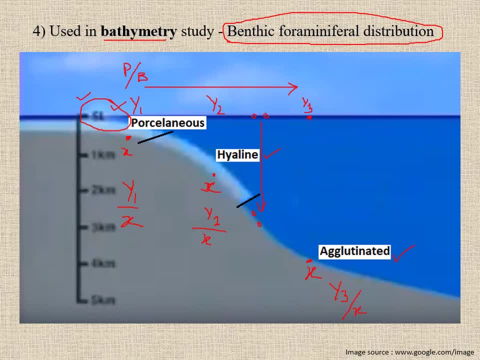 Now as we can, as we know that the number of planktonic foraminifera will increase from coastal areas to open marine areas. so definitely, y2 is greater than y1 and y3 is greater than y2.. So, gradually, from y1, y2 to y3, numbers of planktonic foraminifera will increase. 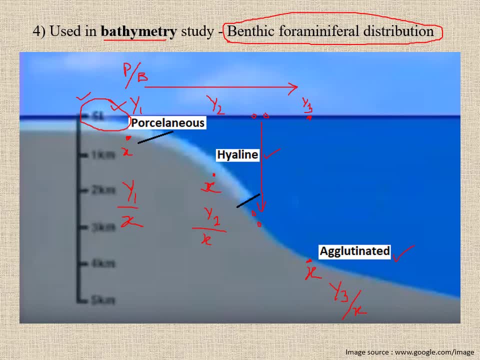 So if we look at this ratio, this planktonic by benthic foraminifera, So always the numerator, that means the planktonic foraminifera numbers will be higher as we move from coastal to open marine areas. So we can say that the planktonic by benthic foraminifera ratio is also increasing as we 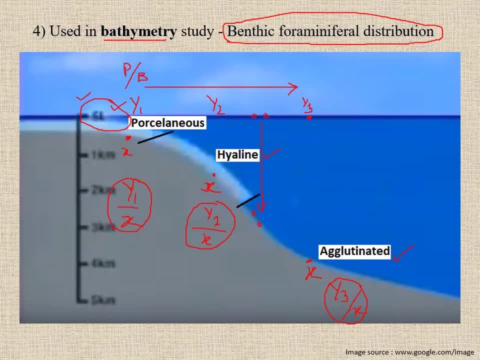 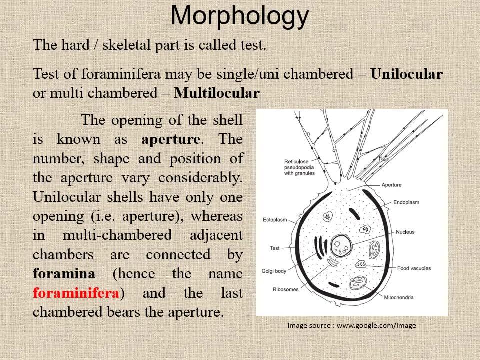 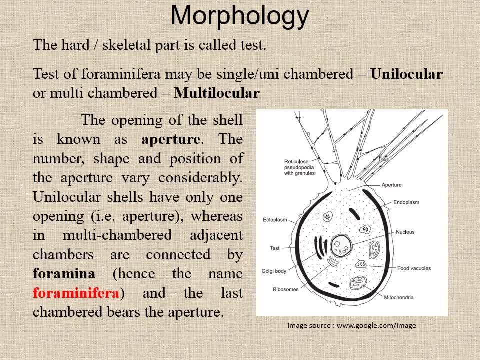 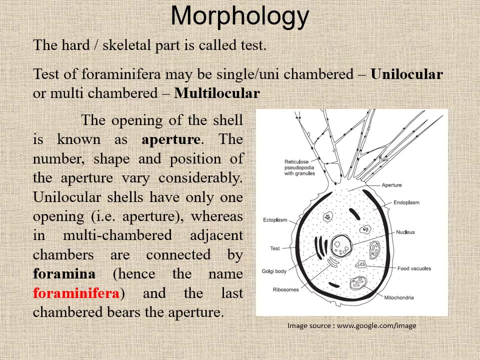 Here we can see this dark colored band. this is the hard part that is made up of test and the cytoplasm Within this cell unicellular body that is occurred inside the hard part as well as outside the hard part. So the inside portion of the cytoplasm occurs within the test that is known as endoplasm. 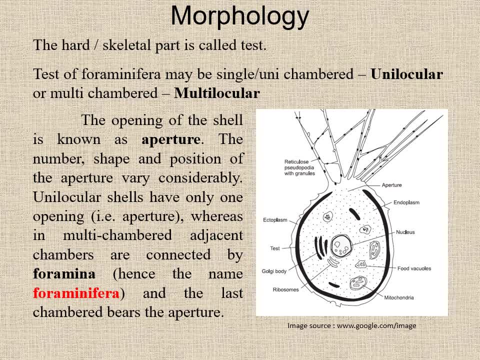 whereas the cytoplasm occurs outside the test, in it as a thin cover that is known as ectoplasm. The test of that is the hard part of foraminifera cells. they may be single chambered or unichambered. 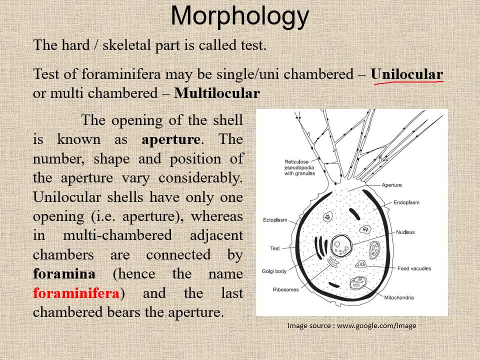 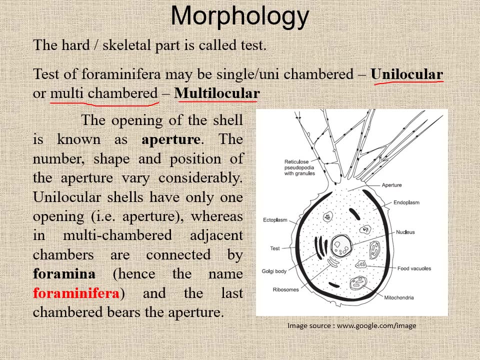 in that case locular, whereas the foraminifera test may be multichambered also. that means they have more than one chamber. also. in that case we call them as multilocular. In this case you can see that the entire foraminifera test having one single chamber. 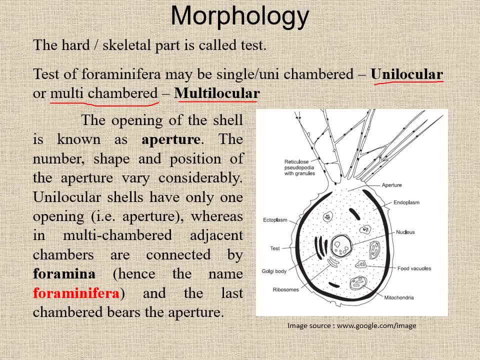 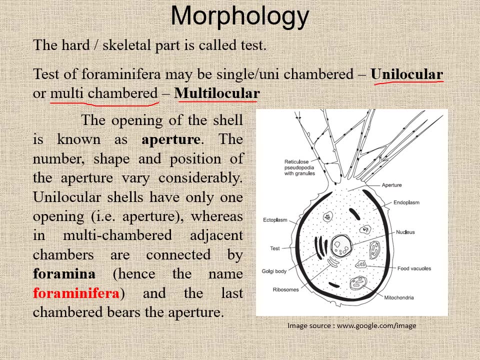 one single place where all the cell materials are occurring. So this one is unilocular. but there are many forms where you can see different or more than one kind of chambers having different shape and size. also Those are called multilocular. 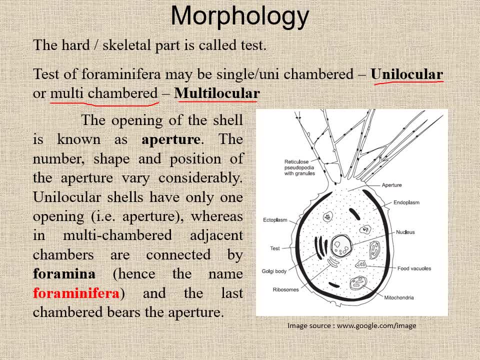 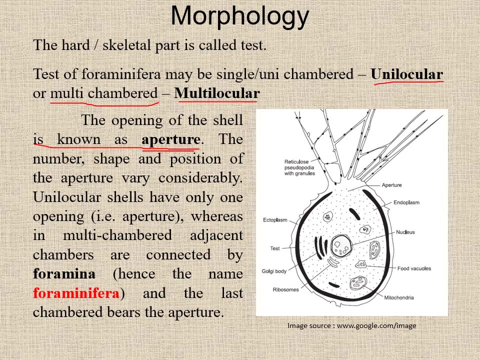 The opening of the cell or more precisely, for the multilocular forms, the opening of the last chamber, is known as the aperture. The number, shape and positions of the aperture vary considerably. So, apart from the main aperture, which is occur particularly for the multilocular forms, 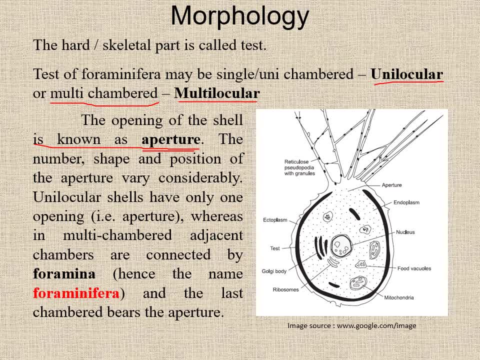 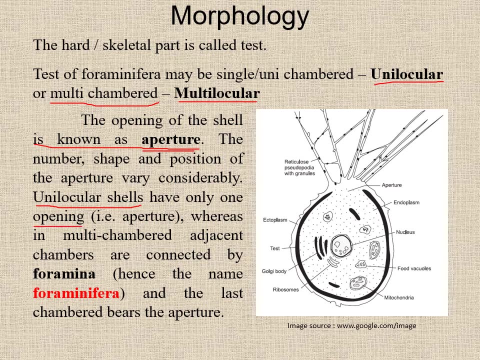 in the last chamber. there are other accessory apertures also, But for unilocular cells, that is, those cells which have only one chamber, they may have only one opening, only one apertures. Apart from the aperture, the multichambered or multilocular foraminiferal cells, they 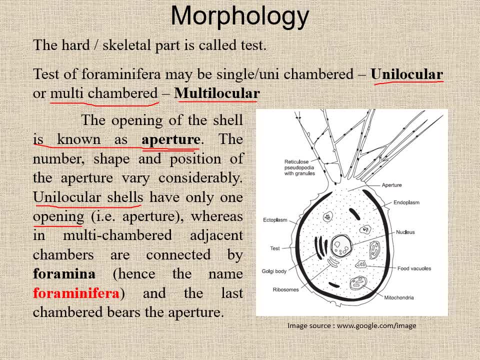 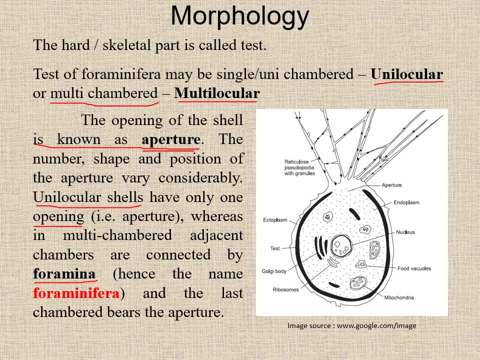 are connected by an opening, which is known as foraminifera, through the different chambers. So all the chambers are connected through an opening, And that opening is known as foramen. Singular number is foramen and in plural number it is known as foramina. 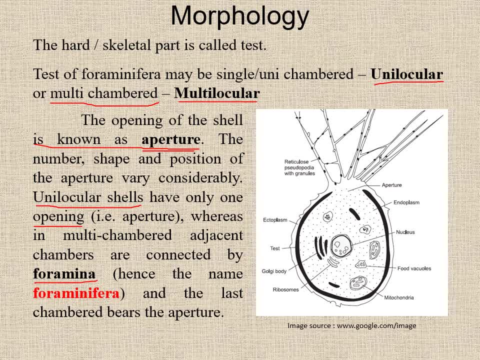 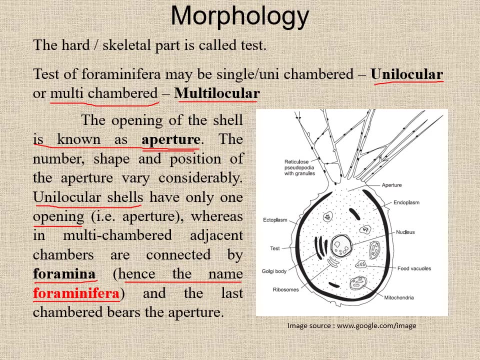 And from these holes, from these foramina, the name of the group of the organism comes, and it is foraminifera. So basically, foramen looks like: suppose this one is a chamber and this one is the above chamber. So here you can see two chambers, two places which are separated by a wall, and within that, 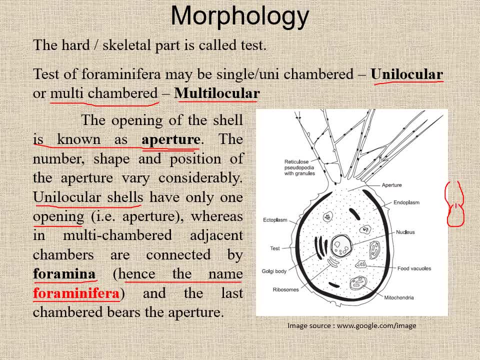 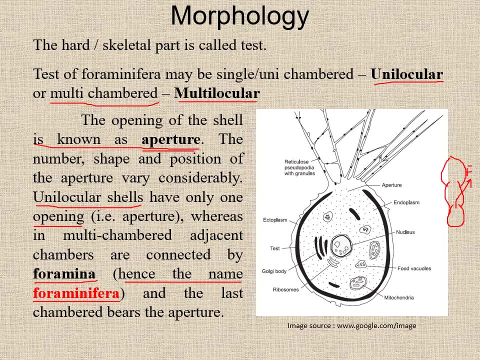 wall there is a hole. This hole is known as foramina, foramen For single. it is foramen If there are multiple number of holes with successive chambers, suppose above this another chamber is there, So again, this one is a hole. in that case, that is foramina. 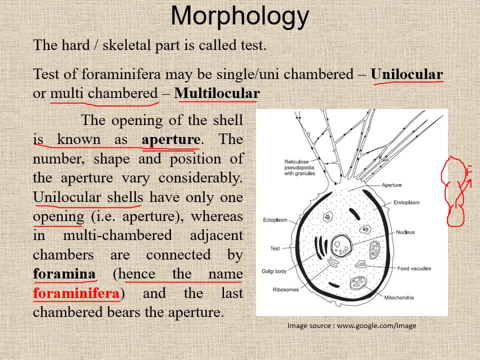 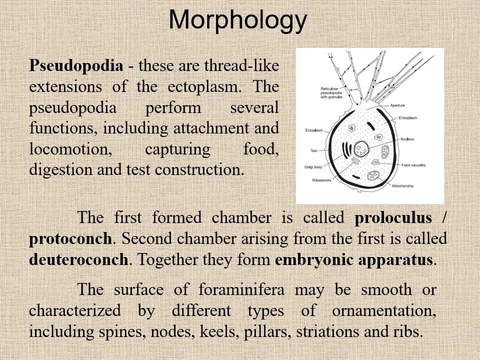 And the organism group having these kinds of foramina. those are known as foraminifera. Now in foraminiferal cells or in foraminiferal organisms We can found that in the frontal part of the aperture there are some thread like extension. 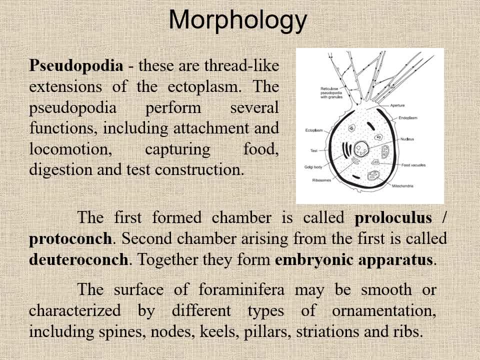 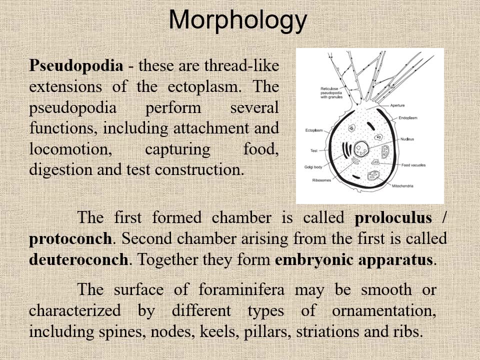 of the ectoplasm, That means the outer cytoplasm. they are extended in front of aperture in some thread like fashion. These are known as pseudoplasm. Pseudoplasm function in a different way. They can act as a attachment. 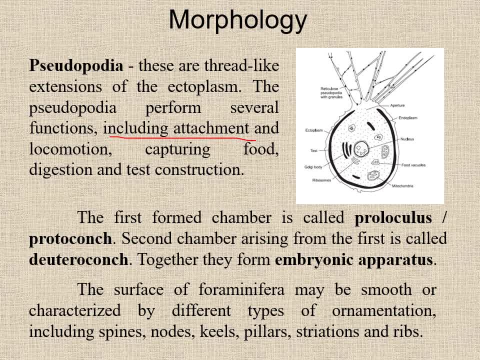 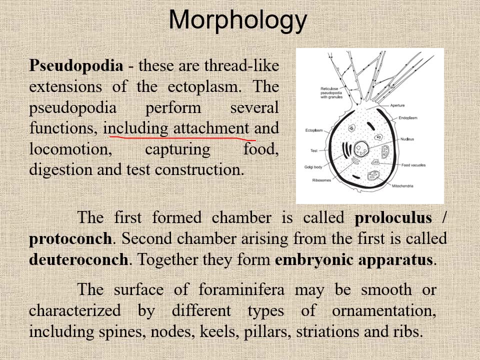 Attachment apparatus. so by functioning the pseudopodia or by using the pseudopodia, the foraminifera test can attach themselves to a hard substrate. These pseudopodia are also act as a locomotory organ. They are also acting as an organ by which they can collect food from the ocean column. 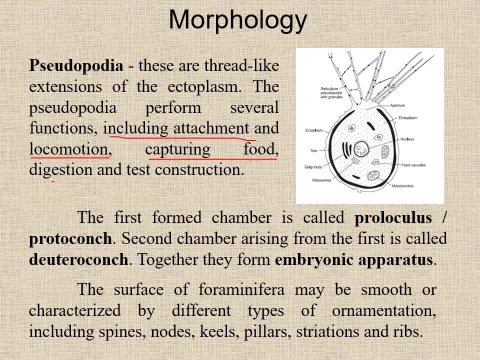 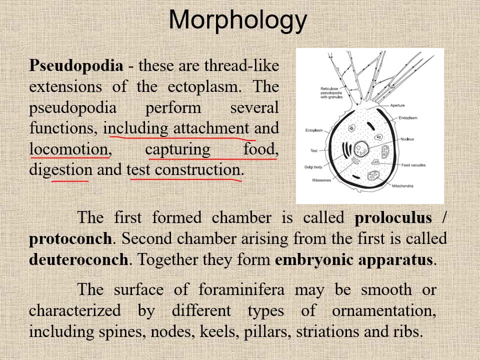 They used for digestion and also they used for test construction. That means hard part material construction also. So you can see that a simple thread like organ is used for different purposes by the foraminiferas. Now the first formed chamber of the foraminifera test is known as proloquilar organ. 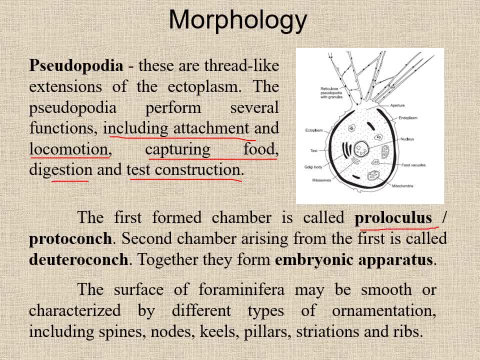 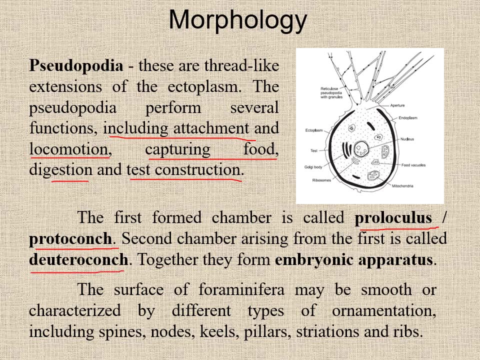 The second formed chamber is known as proloquilus or protoconc. So that is the first formed chamber first formed hard part. The second chamber, formed after the first chamber, is known as deuteroconc. The first one is protoconc. the second chamber is known as deuteroconc. 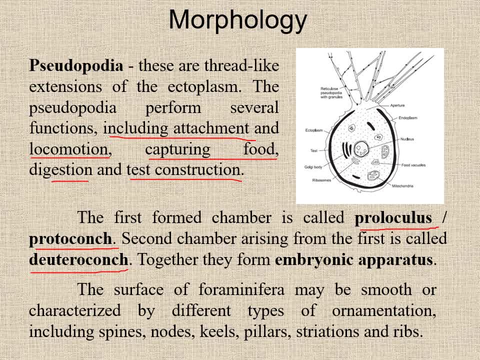 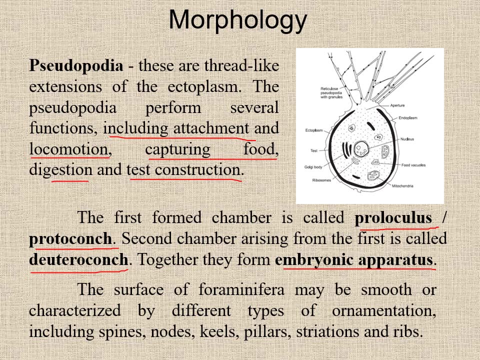 And together this first chamber and second chamber. together they are known as embryonic apparatus. That is, the embryonic stage of foraminifera are restricted within these two chambers. But keep in mind this is valid only where the chamber is multiple. That means for multilocular foraminifera test. 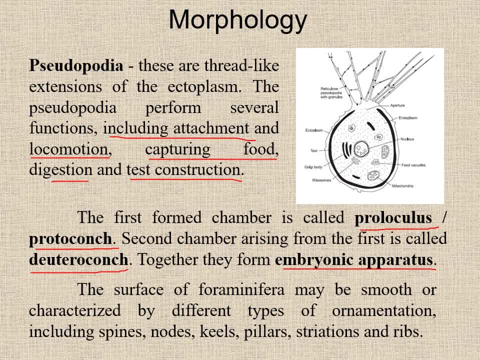 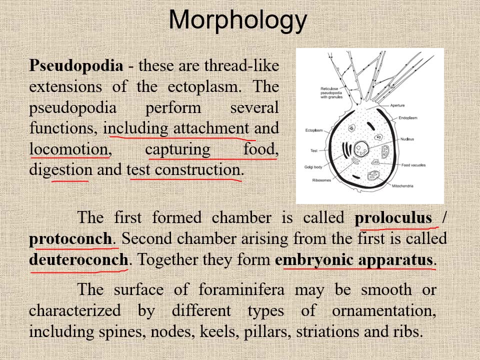 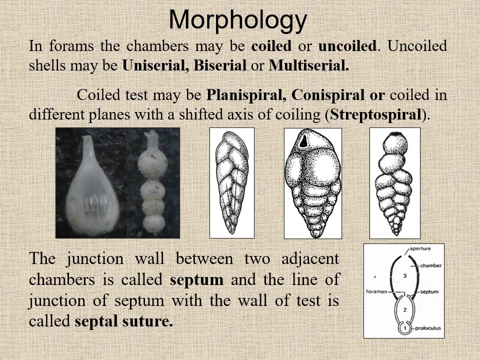 The surface of foraminifera test may be smooth or they may be characterized of different types of ornamentation, Such as spines, Ribs, Like these different kinds. are there Some nodes? are there Kills are there? Different kinds? Now, the foraminifera shells or the foraminifera chambers. they may be coiled or uncoiled also. 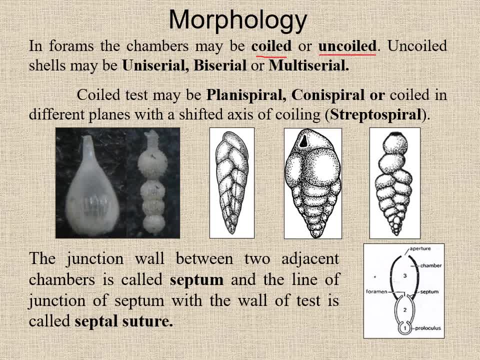 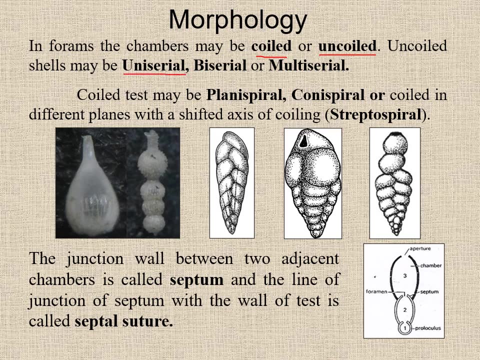 So they may be concentrically arranged around an axis, That is the coiling form, Or they may be uncoiled. also, The uncoiled shells may be uniserial, That is, they are arranged in a single row, In a single series. 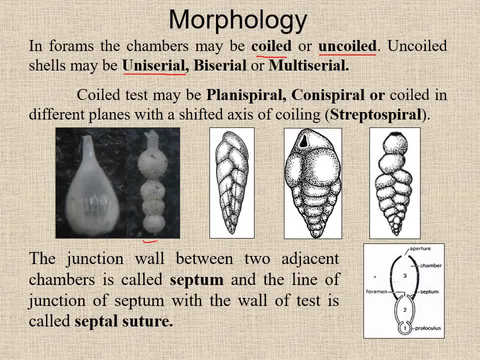 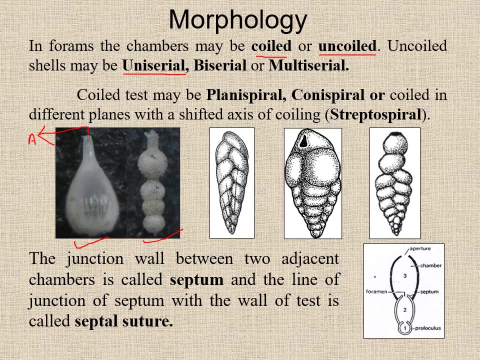 Like this one. You can see that the first picture is of unilocular, That is, unichamber. This one is the aperture, The opening of the chamber. This is the aperture. In the second picture you can see that this is multiple chambers. 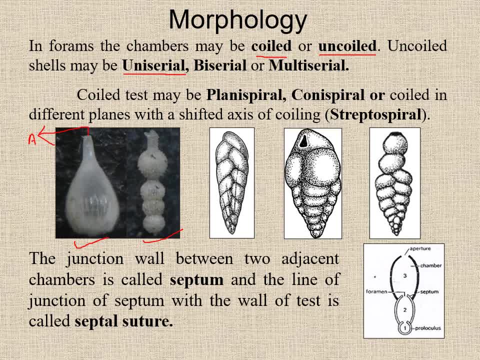 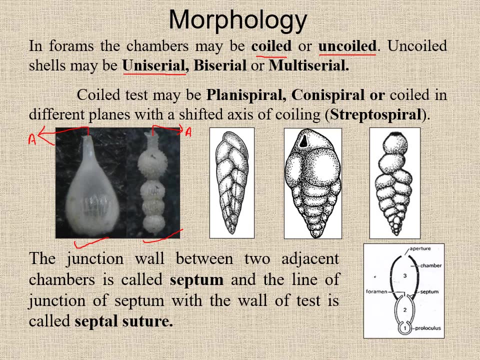 And with ontogeny, the chambers are increasing in size. The opening of the last chamber is the primary aperture. And all these chambers, they are arranged in a series, In a single row or in a single column, So these are uniserial. 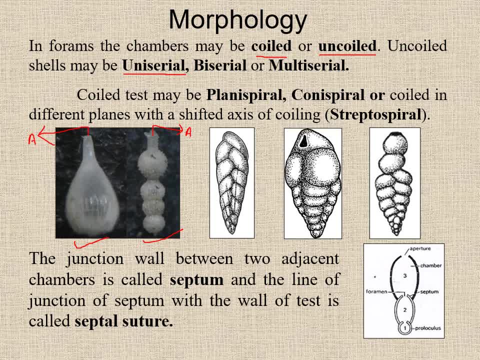 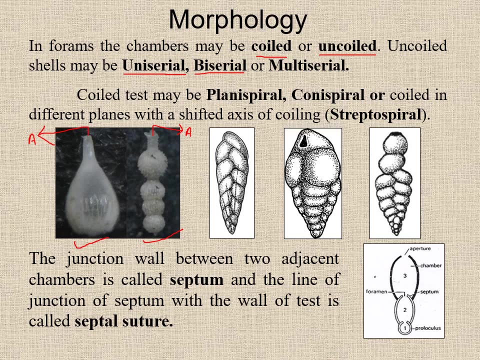 The next type. here you can see, the chambers are almost alternating, arranged In two rows or in two series. These are biserial, And here you can see, the chambers are arranged in more than one series, In more than one rows. Here it is multiserial. 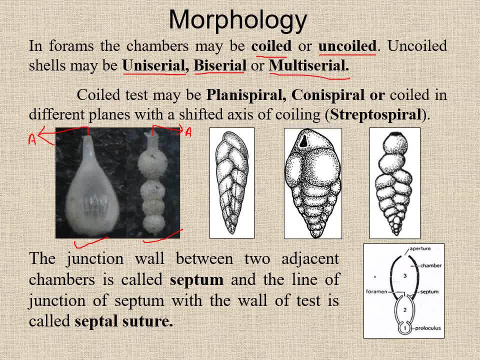 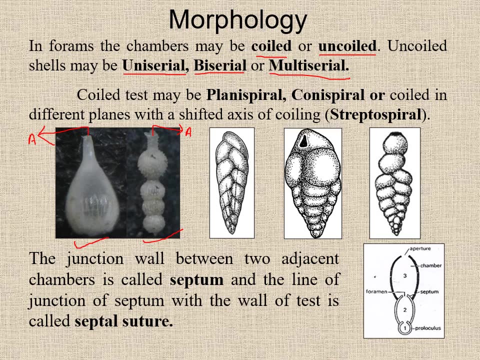 But keep in mind, these are not coiled form, These are not regularly coiled around axis, Only the uncoiled shells. they have these uniserial, biserial and multiserial arrangement And it is often found that the multiserial forms. 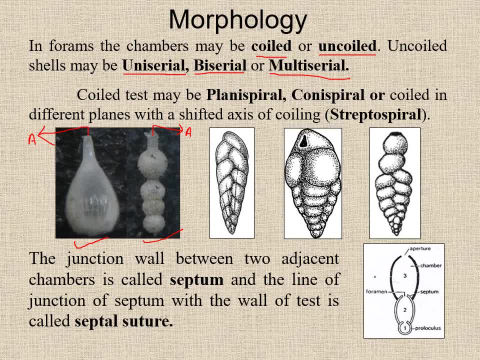 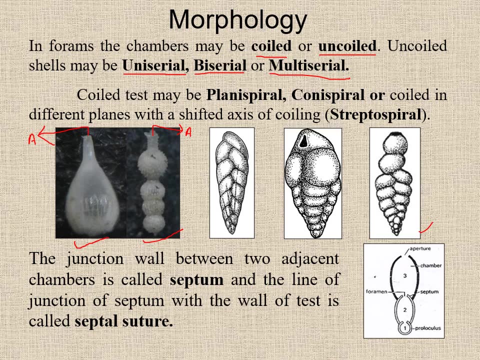 The multiserial foraminiferous shells. They change their series or they change their rows through ontogeny, Say, for example. in this case, You can see that in the earlier stage, in the juvenile stage, The foraminiferous Test is triserial. 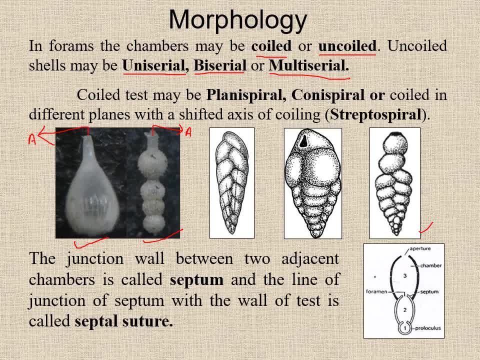 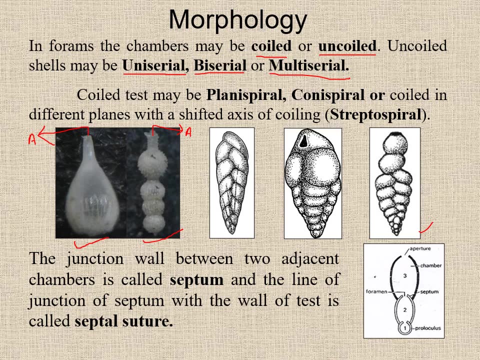 You can see three series of, or three rows of chambers. In the middle stage of its ontogeny, You can see that there are two series of chambers, Two rows of chambers. That is biserial. And in the adult stage, In this last portion, you can see only one chambers arranged in a one series. 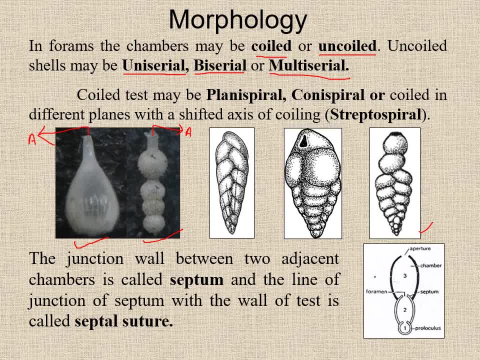 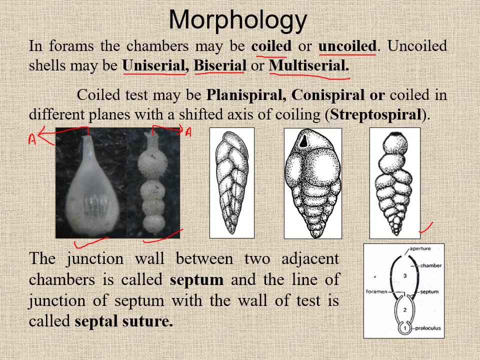 So that is uniserial. So here, Throughout ontogeny, The foraminiferous test changed from triserial to biserial, to uniserial. These kinds of patterns of or these kinds of arrangement of chambers In the uncoiled foraminiferous shells are also found in nature. 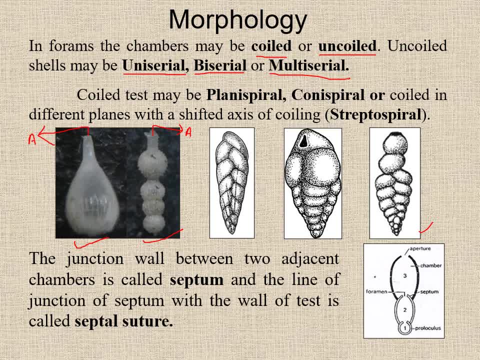 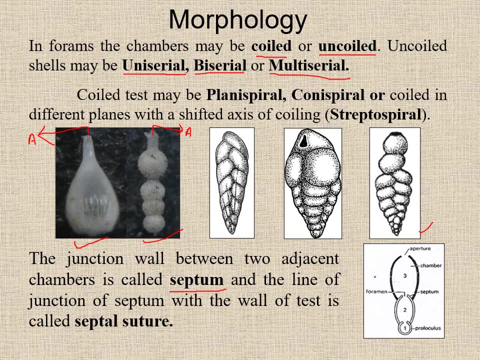 Now the junk chambers Is known as septum. It is almost the same as you learn in the cephalopod. In cephalopod also the dividing wall between two adjacent chambers, Or between two adjacent chmeri. We call them as septum. 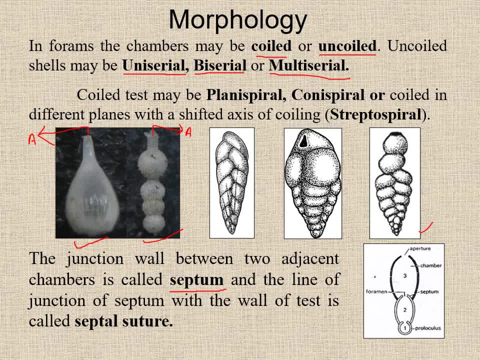 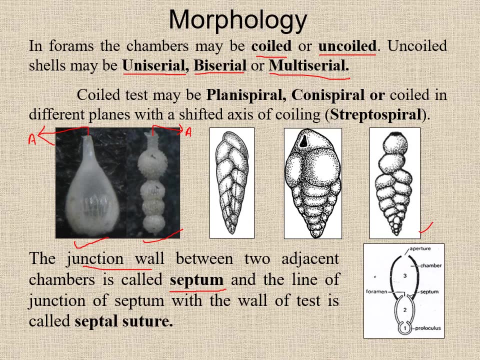 Here also, The junction wall between two adjacent chambers is called as septum. Here you can see This one is the septum And in the septum there was a opening. That is the place by which cytoplasm can move From one chamber to another chamber. 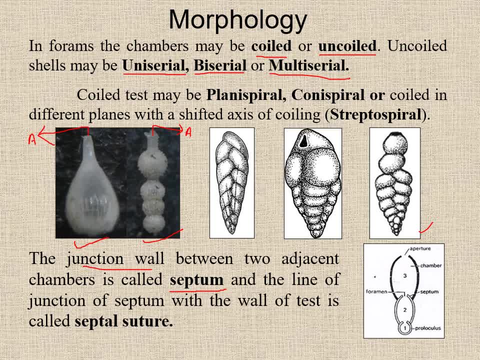 And this opening is known as foramen. If this opening foramen is present in multiple chambers, Here you can see: From three to two there is a one foramen. From one to two there is another foramen. So that means: 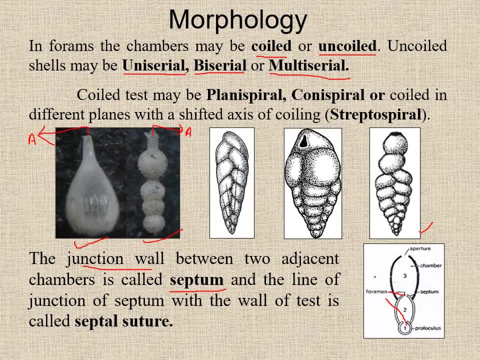 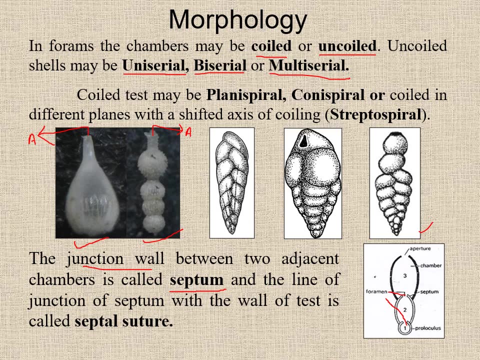 It has multiple number of foramens By which multiple chambers are joined with each other. So these are foramina. Now The septum is connecting or is contacting the shell, the test, along a line, And this line of junction between the septum and the test is known as septal suture. 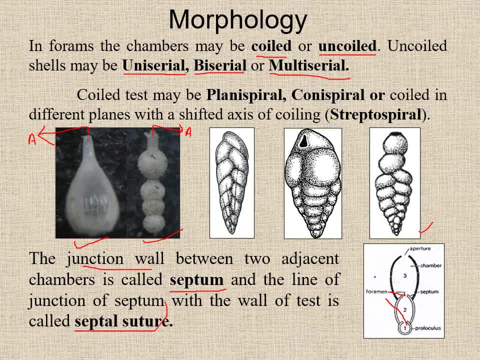 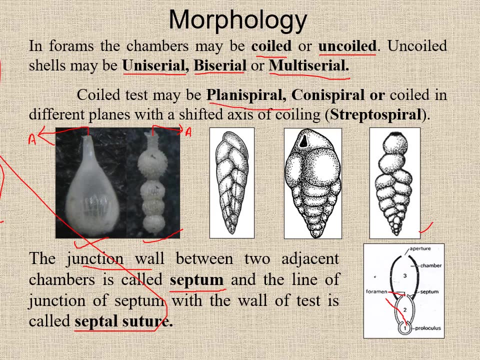 The suture of the cephalopods, Now The coiled. They may be plenispireally coiled, That means coiling occur within a single plane, Or they may be conispirally or trochospirally coiled. 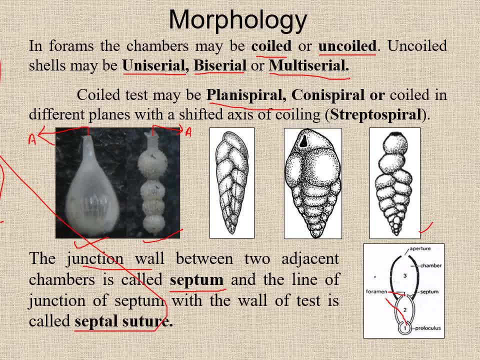 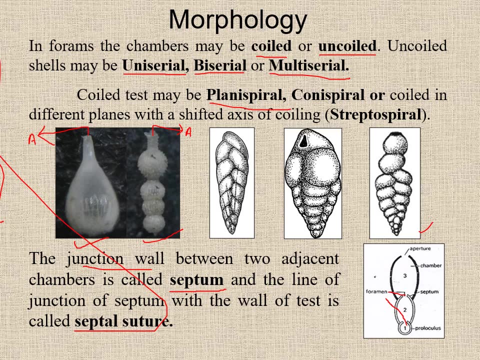 That means coiling occurred with changing plane. That means as the coil occurs, The plane of coiling changes with coiling. And the third type in which the coiled occurs in different planes, And so this portion is similar to the conispiral or trochospiral coiling. 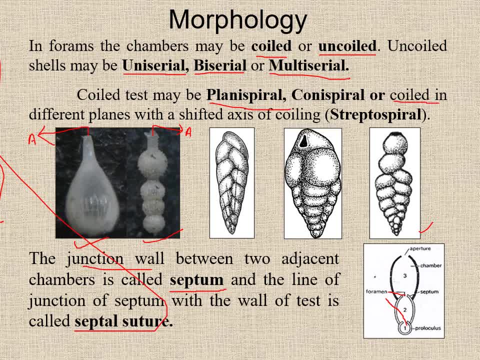 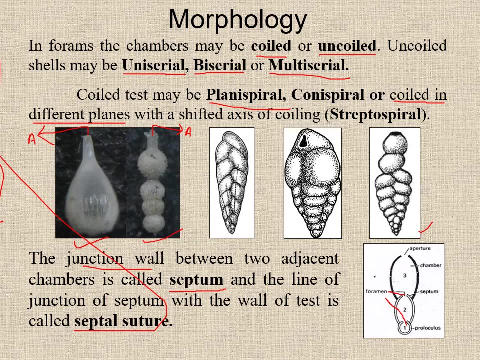 That means coiling occur in different planes. But the difference of conispiral coiling and this streptospiral coiling is that In streptospiral coiling, With changing plane, With changing, With further coiling, The coiling axis is also changed. 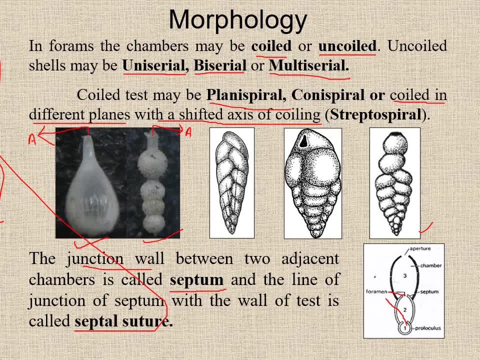 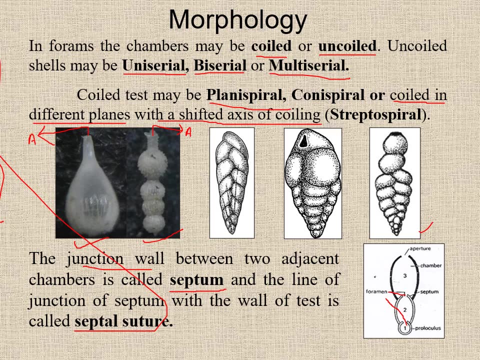 Where, with changing coiling plane, The coiling axis change. That means the axis shifted In different plane In different angles. That type of coiling is known as streptospiral, Now this coiled test. They have also these kinds of septum and septal suture. 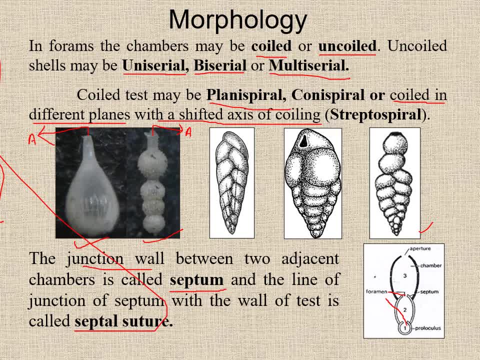 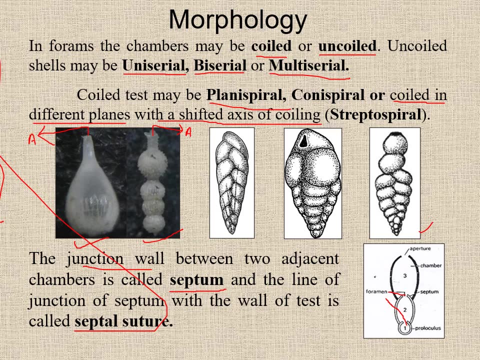 Which have, Which are either coiled or uncoiled. If they have multiple chambers, That means multilocular forms. They bear the structure Here, the septum And the septal suture also. But keep in mind, In encephalopodes 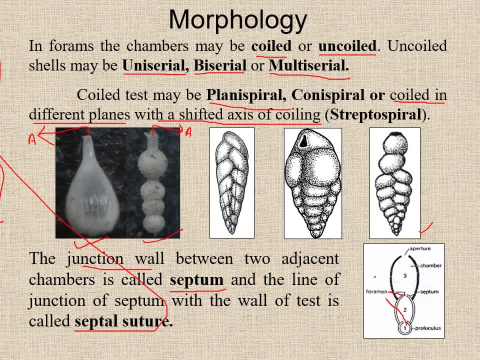 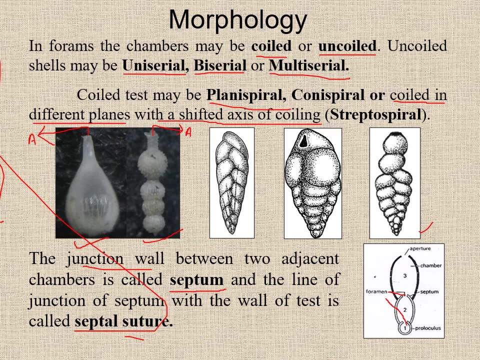 We are all. We are only using the term suture, But in case of Foraminiferal, We are using Septal suture To indicate The junction line joining the septum. And the test Now The reproduction process of 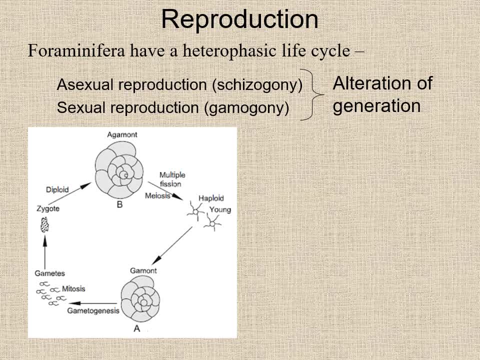 Foraminiferal cells Or foraminiferas Are one of the. In one stage Or in one cycle Their reproduction is done asexually- We call them as Cisogony- And at other time The reproduction process is done by sexual way. 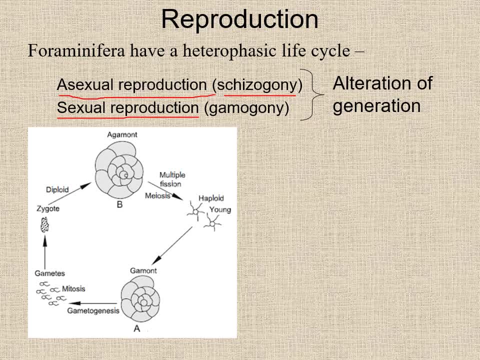 And Process is known as Gamogon. So In a complete cycle You can see In this half From This one. When reproduction occurs By haploid processes And meiosis type of cell division, This process is done by asexual reproduction. 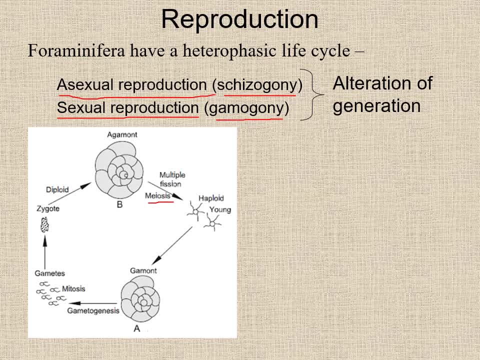 Gamont, Whereas from gamont They reproduce sexually By mitosis type of cell division. By producing gametes And zygotes Through the Sexual way And gamogony process of reproduction, They will produce the Product. 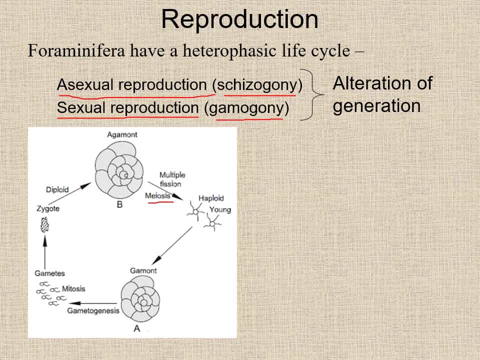 These Gamonts, Their first form chambers, Is very large Compared to the Relative Sizes of other cells. So The Proloquilus is large sized, But the Endocrine Is very large, So The 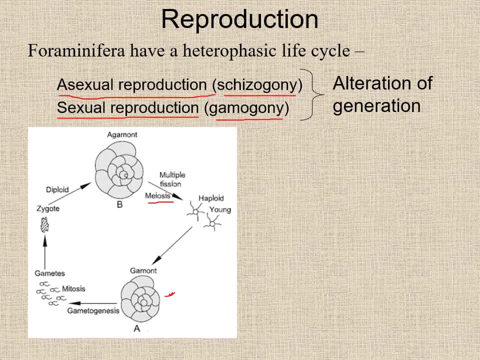 Proloquilus Is very large, But the Endocrine Is very large, So The Entire Cell Is smaller in size. So This Gamont is, Or this Product Is also known as, Megalospheric. 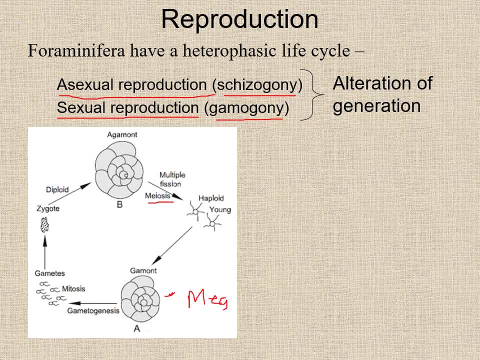 Because They have A large Proloquilus. So, Depending On this Mega Size Of Proloquilus, The This Gamont Individual Which is Produced By Asexual Reproduction. 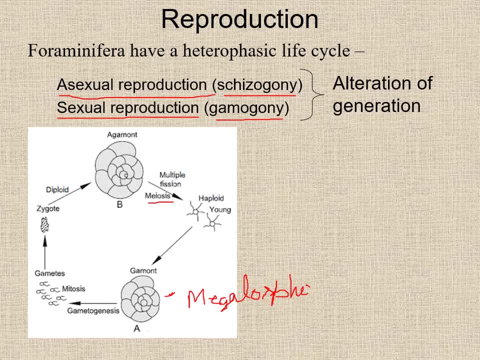 They Are Known As Megalospheric Test In Contrast The Products Produced By Sexual Reproduction, By Mitosis, Type Of Cell Divisions, That Is, By 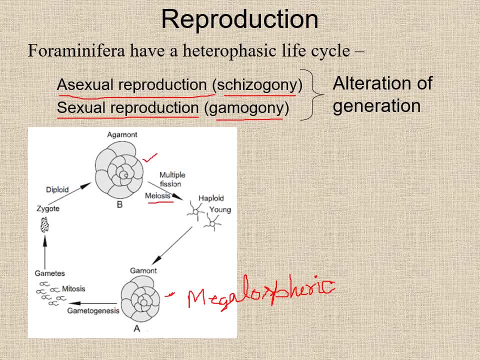 Gamogony. They Have A Size Compared To In Gamont. You Can See In Gamont The Proloquilus Is Very Large But The Entire 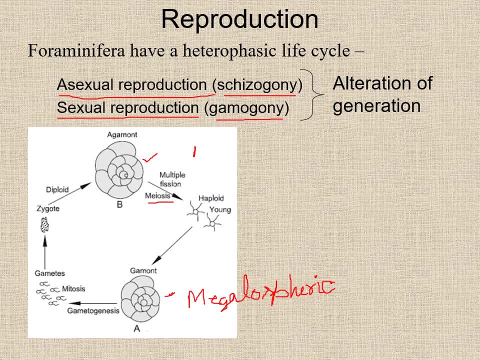 Cell Is Relatively Smaller, But In Agamont In Gamogony Process The Individuals. This Type Of Individual Cells Is Known As Microspheric, So 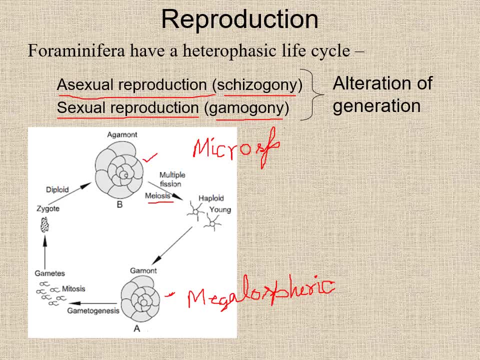 All These Megalospheric And Microspheric Terminology Are Named And Given Depending On The Size Of The Proloquilus. Keep The Size Of. 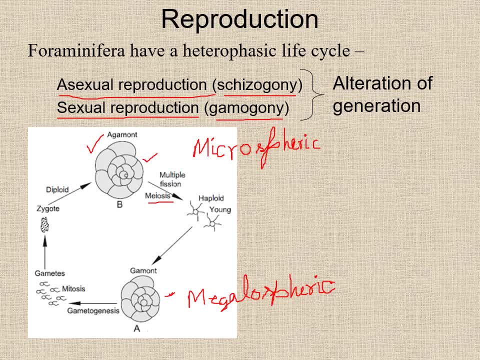 The Cell In This Agamont Is Always Larger. Cell Size Is Greater Compared To Gamont In Agamont Individuals But Proloquilus Size Is 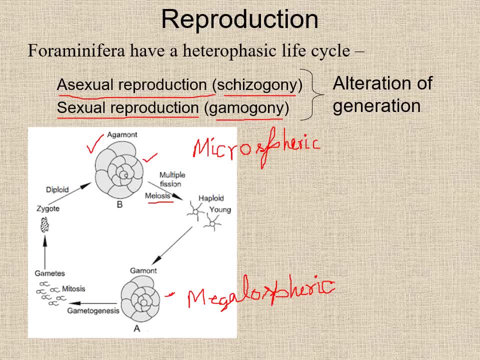 Larger In Gamont Compared To The Size Of The Cell And The Size Of The Cell Is Larger Compared To The Size Of Gamont. And. 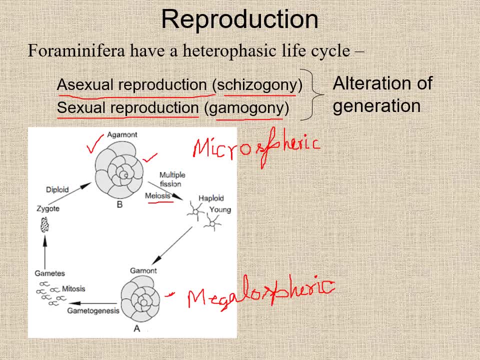 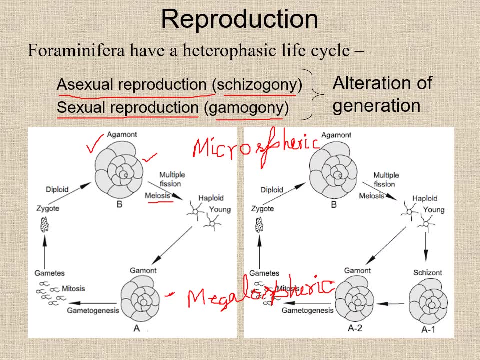 The Size Is Larger Compared To The Size Of Gamont And The Size Is Larger Compared To The Size Of The Size Of Gamont, And. 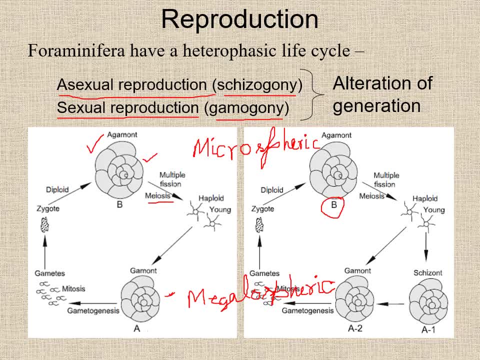 The Size. Of The Size Is Larger Compared Compared To Size Of And this intermediate stage, saizont, is also known as A1 form, and from this saizont or saizont, the gamont are produced, that is, the A2 form, and from this gamont by sexual reproduction. 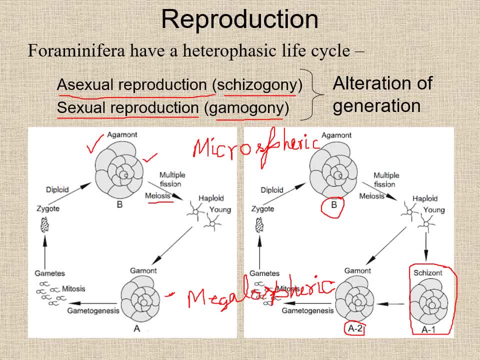 way the agamont is produced, which is the B form. So here, according to some authors, according to some scientists, in the entire reproduction process of foraminifera, we get three morpho variations or three varieties of foraminifera test: the agamont, saizont and gamont.